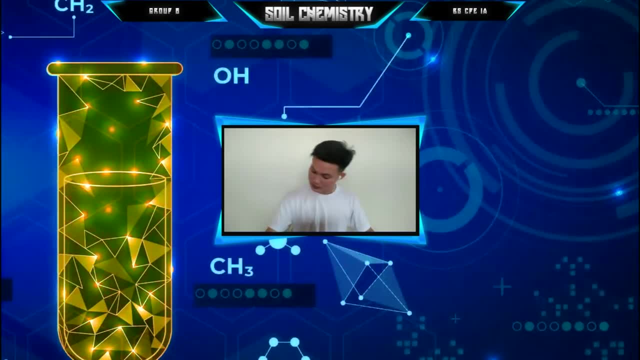 You can also connect your phone at the address given in the video description. You can also connect your phone at the address given in the video description. Hey guys, welcome back to our stream. And so for today's video, I am very interested to discuss something interesting and, at the same time, knowledgeable for you guys. 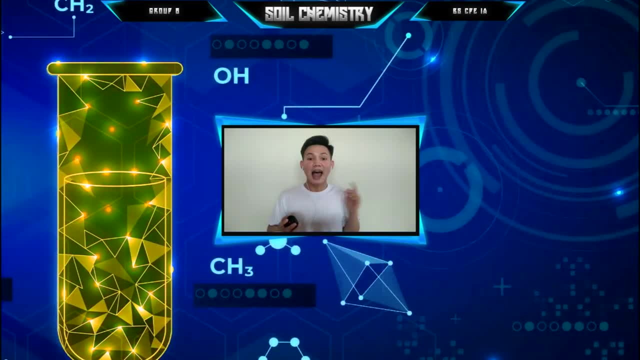 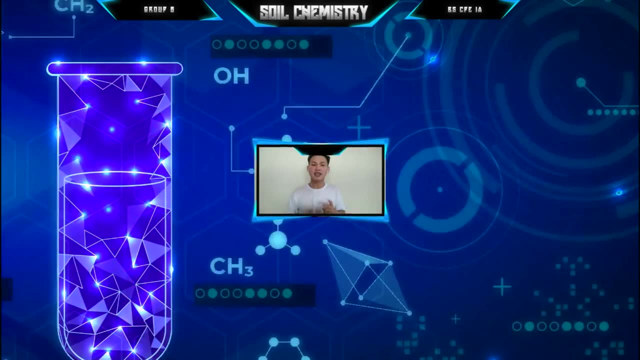 And for today's stream it is kind of special because I am not the only one who is going to discuss something for you today, Because I have my classmate here to help me spread something interesting and at the same time, knowledgeable for you guys. 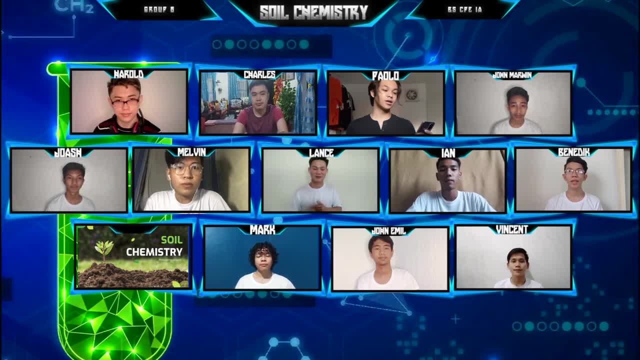 Hey guys, thank you for joining me today. So, guys, how are you doing in this time of pandemic? I hope you are all doing alright, because it's so hard to cope up with stress in school, works and in life. So are you ready to help me discuss something interesting for our viewers today? 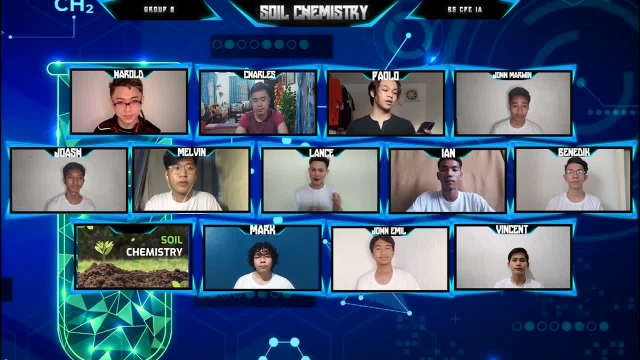 Okay for today's stream. we are going to dig deeper about. Can you guess it, guys? What is the topic that we are going to talk about? Can you guess it? Okay? Okay, you guessed it. We are going to talk about soil chemistry. 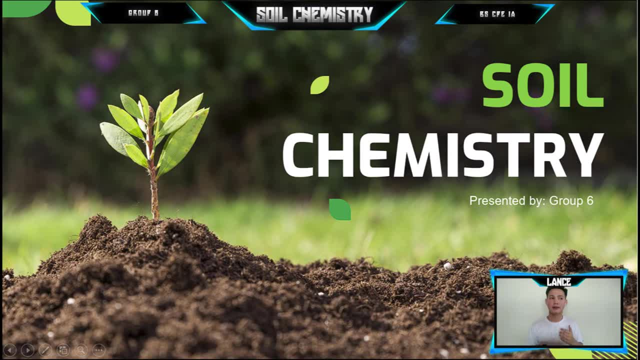 Most of the time, we often take it for granted every time that we found delicious fruits or vegetables in market or in our fridge. However, did you stop and think about it? Where are all these food came from? or what happens in the soil when food is produced? 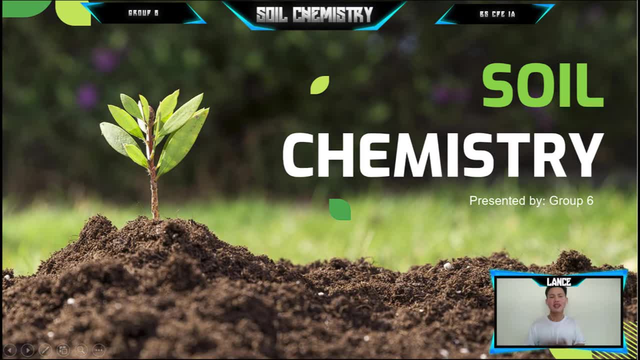 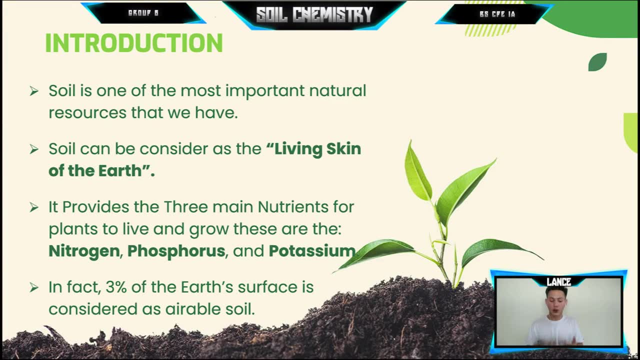 Today we are going to find that out, But first let me define what is soil. Soil is a loose material that covers the earth's surface. in the most part of the world and land is covered by soil. You can think of soil as the living skin of the earth. 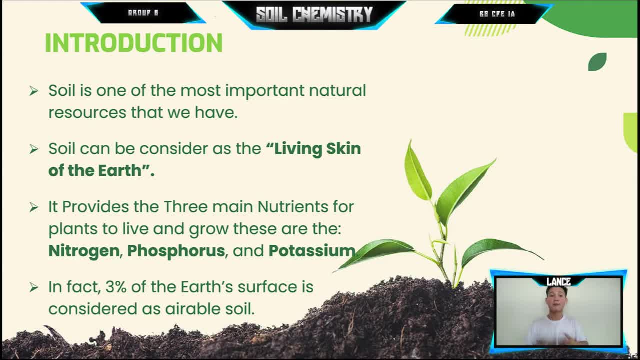 Soil also provide nutrients for plants, for them to live and grow. Soil is a major source of nutrients. Soil is a major source of nutrients for plants, for them to live and grow. Soil is a major source of nutrients for plants, for them to live and grow. 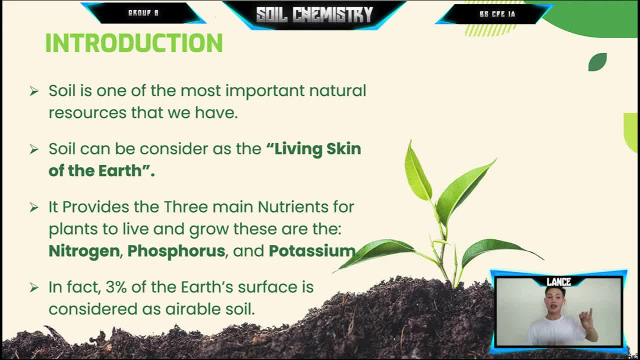 The three main nutrients are: We have nitrogen, we have phosphorus and, lastly, we have potassium. That is why it is very important for us humans to protect and preserve our environment, most especially the soil, Because if we continue doing our wrong habit, which is poisoning our soil, 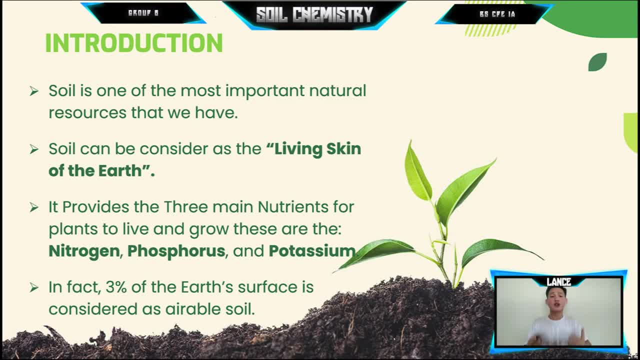 its effect will bounce back to us humans, Because if the soil that we have is poisonous or is not an ideal to plant on, How can we continue doing our wrong habit, which is poisoning our soil? its effect will bounce back to us humans, Because if the soil that we have is poisonous or is not an ideal to plant on, 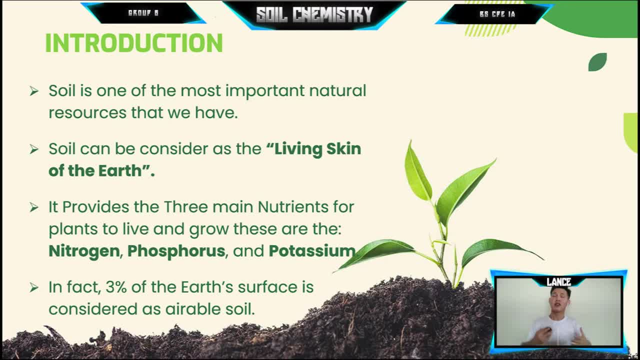 How can we continue doing our wrong habit, which is poisoning our soil? its effect will bounce back to us humans, Because we humans and also the animals, we cannot produce our own food. Only the plants can produce their own food. And if we can't plant our own soil, how can we plant it? 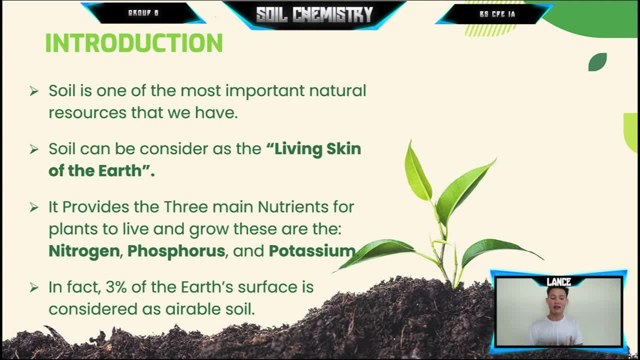 And if we can't plant it, how can we eat it? That is why we need to educate ourselves and, at the same time, we need to have self-discipline. On the other hand, There are things we should be aware of, because we only had limited amount of our soil. 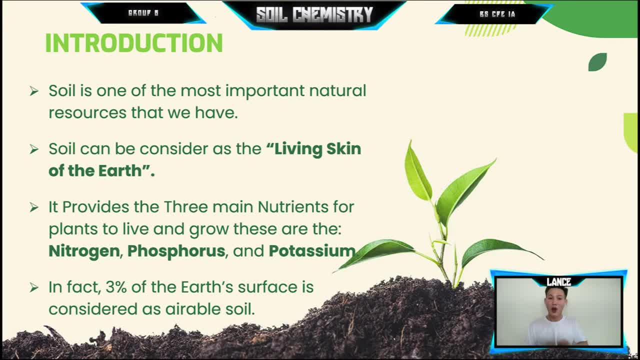 there are things we should be aware of. there are things we should be aware of of arable soil. In fact, only about 3% of the Earth's surface is considered as arable soil. The rest consists of water, cities, swamps, deserts and mountains. 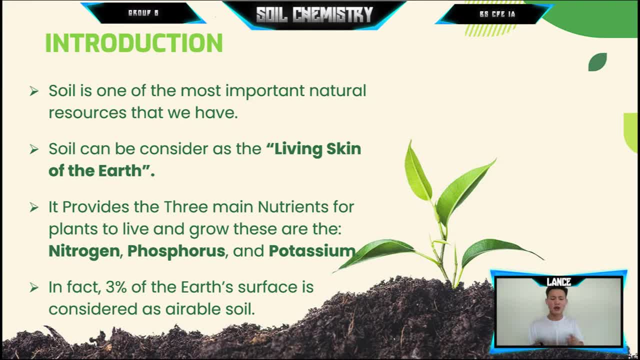 Nonetheless, soil is not just a dirt, because it is an important natural resources on our planet that provides the foundation for the 7 billion life on Earth. On a final note, soil is essential for life. Soil is an ecosystem in which millions of living creatures live and interact. That is why, as humans, it is 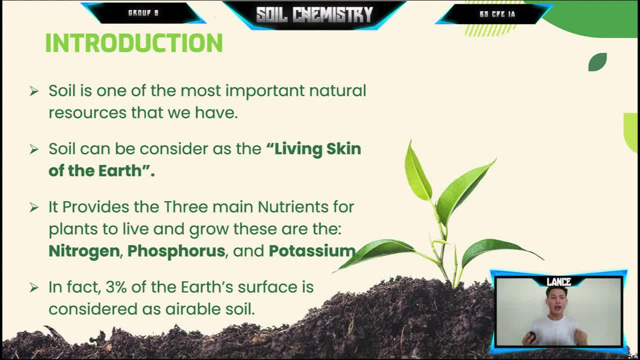 very important for us to remind ourselves why we are here. We are here to protect and preserve God's Creator, so that the next generation may feel and see the beauty of our home called Earth. So next let's talk about soil. Let John Emil Torres discuss the main objective, or the main discussion for 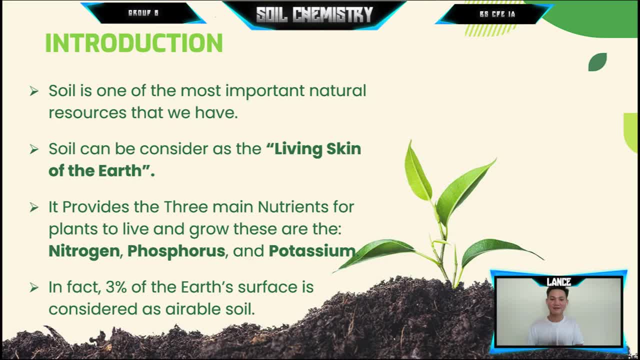 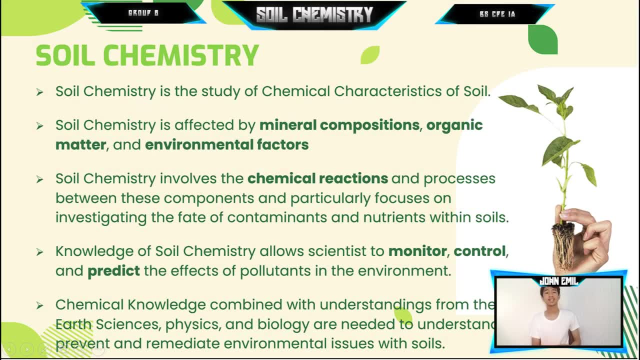 today, which is the soil chemistry. I'm here to discuss the soil chemistry. But first, what is soil chemistry? It is the study of chemical characteristics of soil affected by mineral composition, organic matter and environmental factors. Also, it is the branch of soil science. 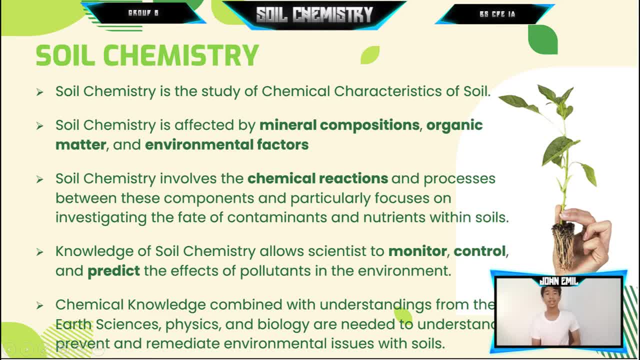 that deals with the chemical composition, chemical properties and chemical reaction of soil In both the chemical reaction in soil that affect plant growth and plant nutrient, and process between the components and particularly focus on investigating the fate of contaminant in the subsurface and surface and also the 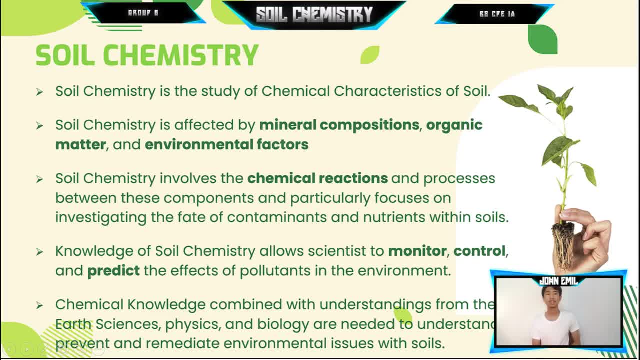 nutrient of soil. To understanding of the chemistry and mineralogy of an organic and organic soil component is necessary to comprehend the area of chemical reaction that contaminants may undergo in the soil environment. Soil chemistry is concerned with the chemical reaction and process involving these phases. 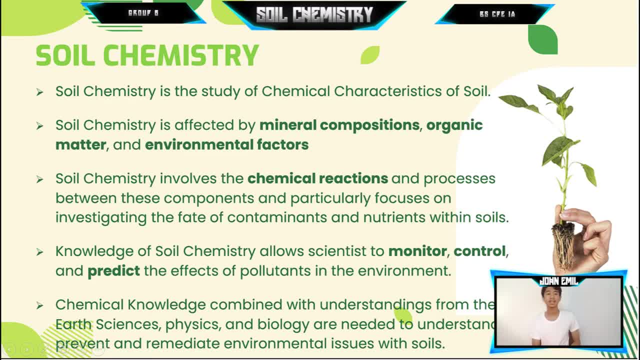 For example, carbon dioxide in the air combined with water acts to weather the inorganic solid phase. chemical reaction between the soil solid and the soil solution influence both plant growth and water quality. Soil are heterogeneous mixtures of air, water and inorganic and organic. 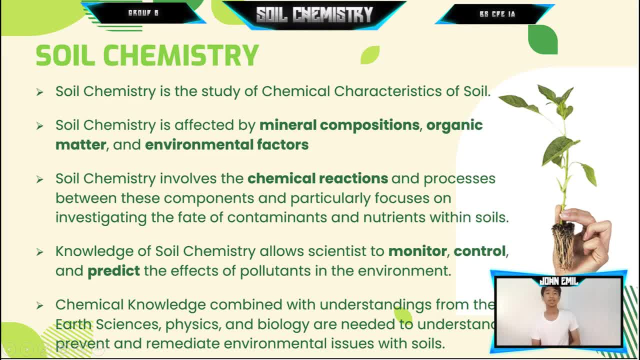 and microorganism. But first, what is the importance of soil? Soil is essential for life. It is an ecosystem in which millions of living creatures live and interact. It is also important to the farmers in planting their crops- vegetables and especially. 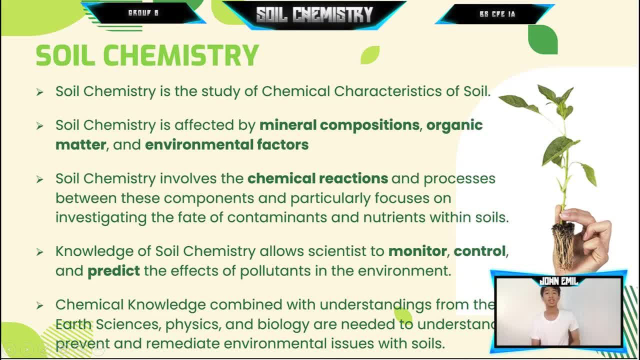 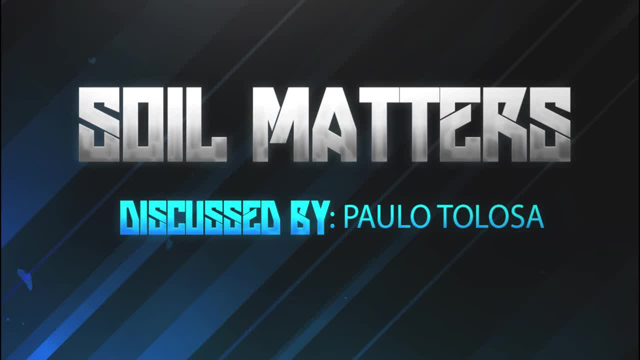 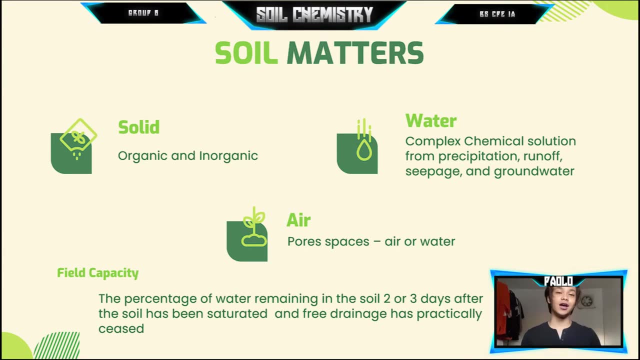 rice, Also in building infrastructure. So now let's Paulo Tolosa discuss the soil matters. Thank you, John Emil Torres. Today I am Paulo Tolosa and we will be discussing soil matters. So first of all, what is soil? Soil is the unconsolidated mineral or organic material on the immediate. 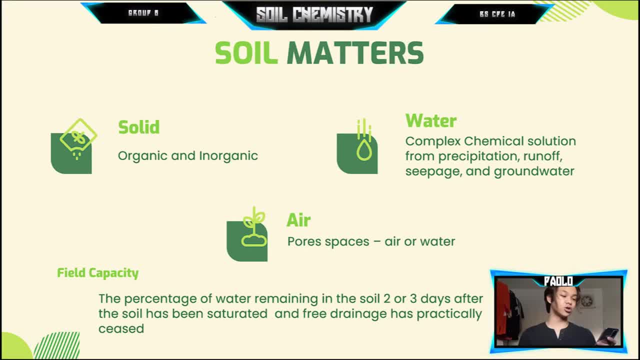 surface of the earth that serves as a natural medium for the growth of land plants. So, as you guys know, soil, soil is everywhere, Like almost everywhere. We need soil in order, to you know, make our plants grow. So, in solid, organic matter is quantitatively a minor fraction of soil In organic solid. 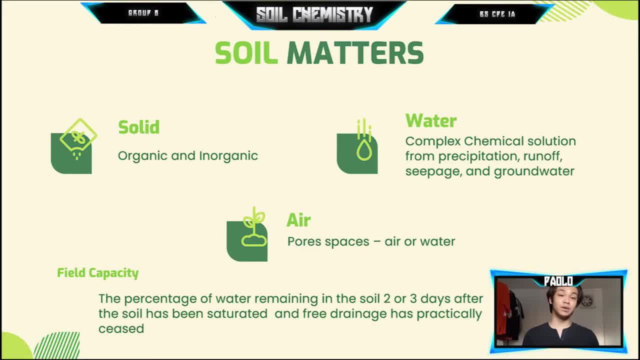 bases in soils can generally be described as minerals. In soils, rock provides the raw, Like you know, soil. it contains rocks and rocks are minerals. So minerals may derive directly from rocks with little or no chemical or structural changes, Although physical changes, like you know, is truly from levels and such more. 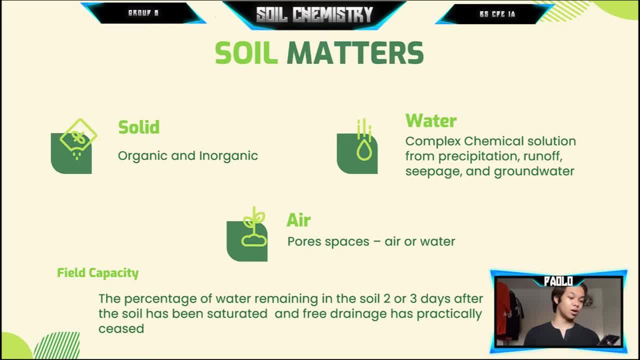 Air Pour space is that part of that volume that is not occupied by either mineral or organic matter, But is open space occupied by either air or water. Ideally, the total pour space should be about half of the soil volume. So it means the airspace is needed to supply oxygen to plant roots and soil organisms. 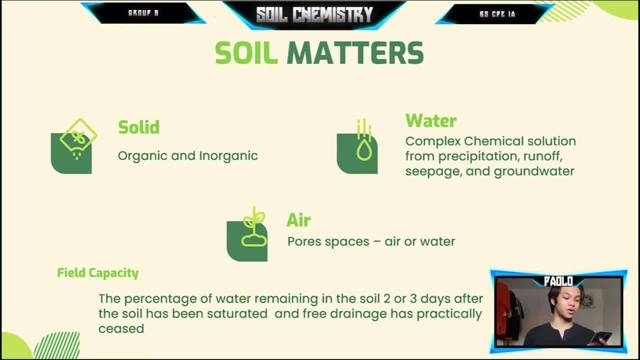 Pore space also allows the movement and storage of water and dissolved nutrients. Next is water. Soil moisture, also known as water content, is the quantity of water contained in soil. Soil moisture or soil water is important as it serves as a carrier of plant nutrients. 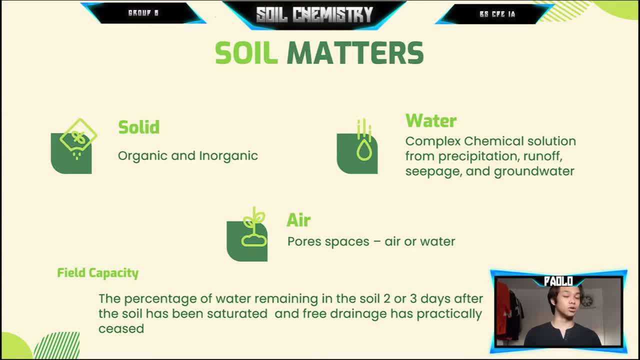 So without water plants won't be able to survive. To regulate soil temperature, those is microbial activity and many more crucial activities that are essential for plant growth. So that's pretty much it, the three phases of soil. So field capacity is the amount of soil moisture or water content held in the soil after excess water has drained away. 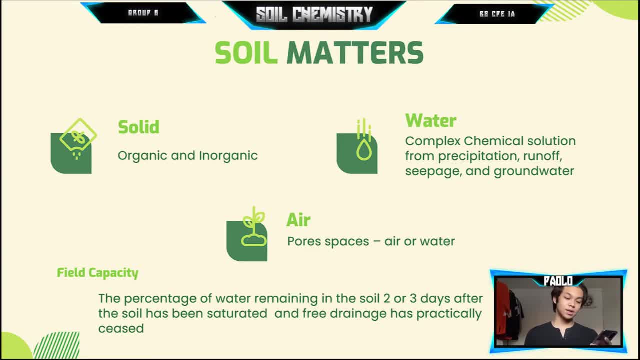 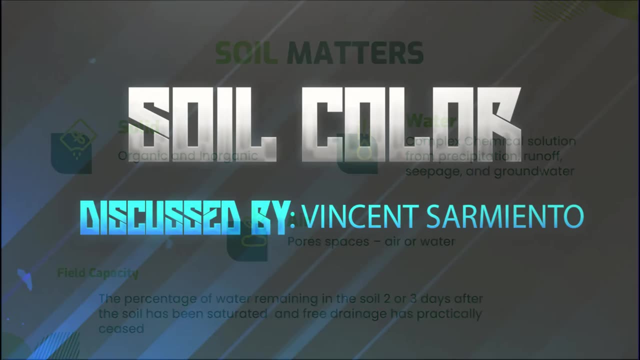 and the rate of downward movement. This usually takes place 2-3 days after rain or irrigation in previous soil of uniform structure and texture. Furthermore, let's call on Vincent Sarmento to discuss soil color. Vincent, What do you mean by soil color? 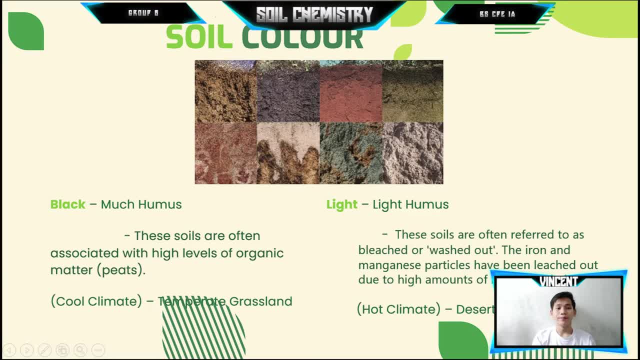 Soil color tells us stories on how the soil is formed. The first impression we have when looking at soil color is the soil color of the plant. Soil color is the soil color of the plant. Soil color is the soil color of the plant. at bare earth or soil is colors of bright colors especially catch our eye and soil can vary with. 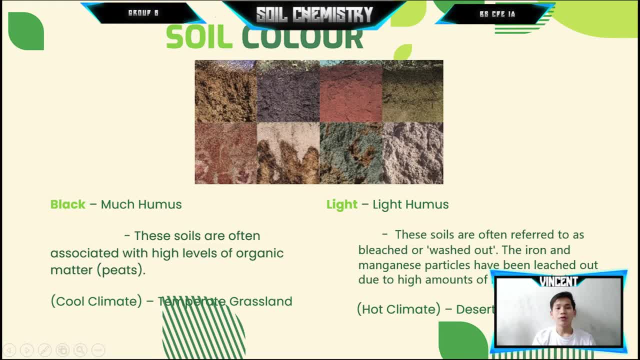 ecosystem, the story of soil color tell us, vary with the ecosystem in which the soil form and are influenced by parent material and some other factors. soil come in different shades. most shades of soil are black, brown, red, gray and white. now let's discuss the different types of soil color. let me begin in clear or white soil color. they may be white, from which they 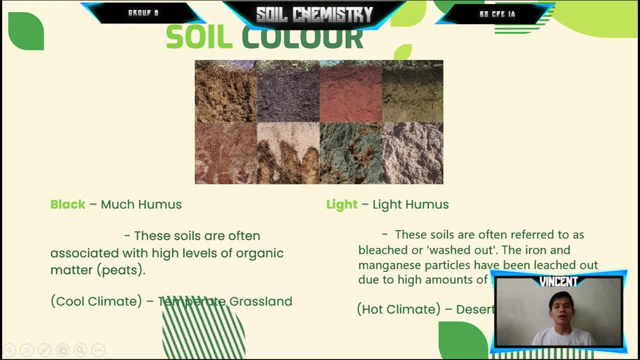 may be influenced by calcium and magnesium carbonates, gypsum or other more soluble salts, often a white layers, mostly quartz. of course, between organic matters on the surface where pigments were removed will consist state soil. secondly, the brown soil color brown, so it might be brown from decaying plant material. the darker color often indicates and they compose organic. 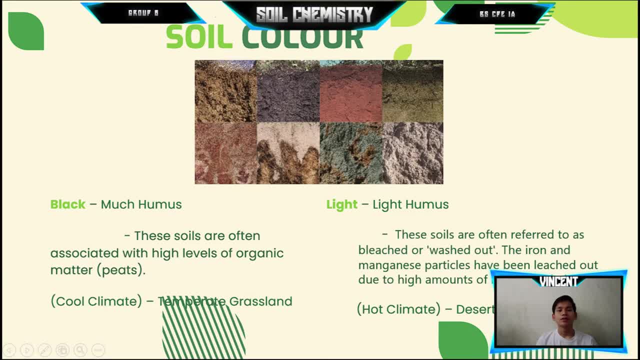 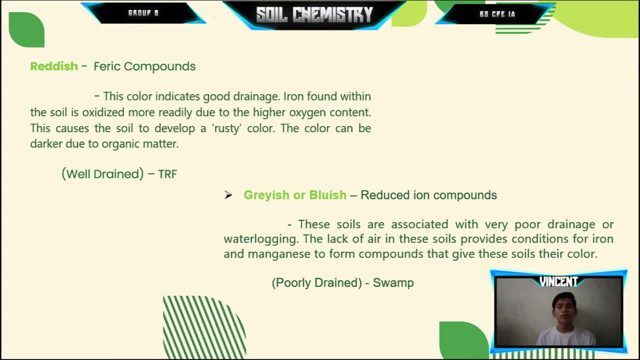 matter know as humus, soil has living or organism and then organic matter which decompose into black humus. the third one, yellow or red soil colors. yellow or red soil indicates the presence of oxide parent iron oxides. the red color might be mainly due to pair of sides occurring as a thin coatings on the soil particles. 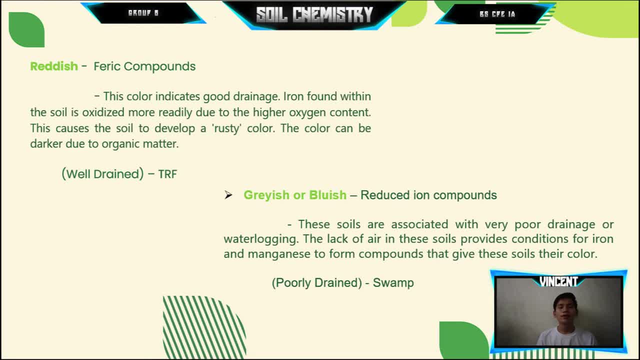 while the iron oxides, of course, as a hematite or a hydrospheric oxide, the color is red and when it occurs in the hematite form, as limonite, the soil gets a yellow color and, lastly, gray soil colors. organic matter plays an indirect but crucial role in the removal of iron and 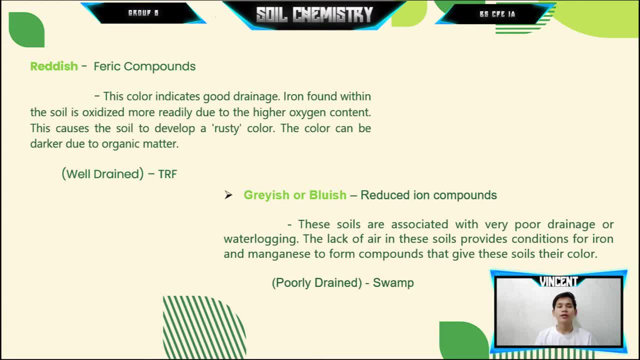 and, lastly, gray soil colors. organic matter plays an indirect but crucial role in the removal of iron and in manganese pigments in wet soil. all bacteria, and DDR Bahria, including those that reduce iron and manganese, must have a food source that a very painful, therefore anaerobic bacteria. 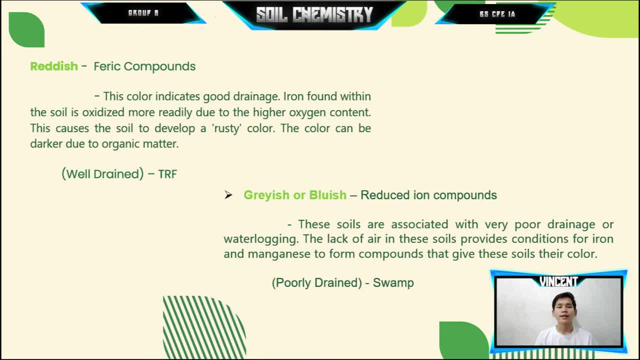 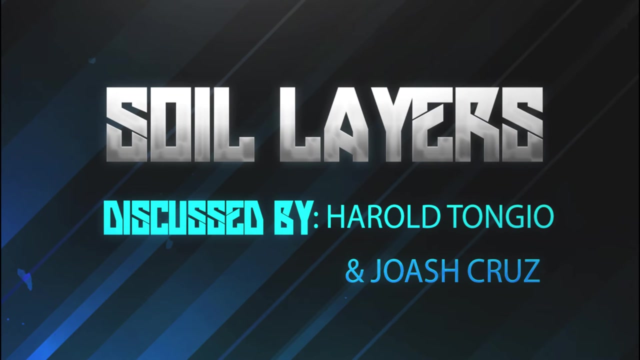 died in concentrations of a organic matter, particularly in dead root. that's the soil's colors. and now let's move on the soil layer to be and discussed by, harrell tonguial and Jowash Cruz. Hello guys, I'm Jowash Hernandez Cruz and I'm going to discuss the soil layer. 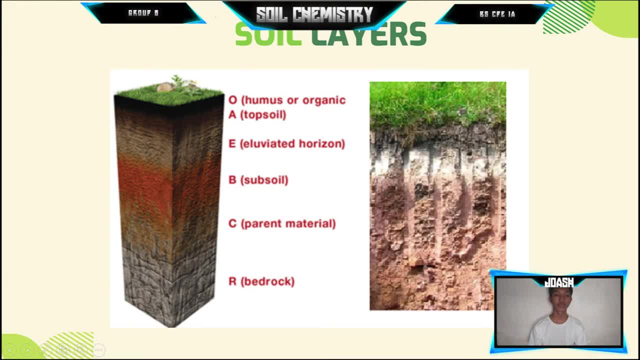 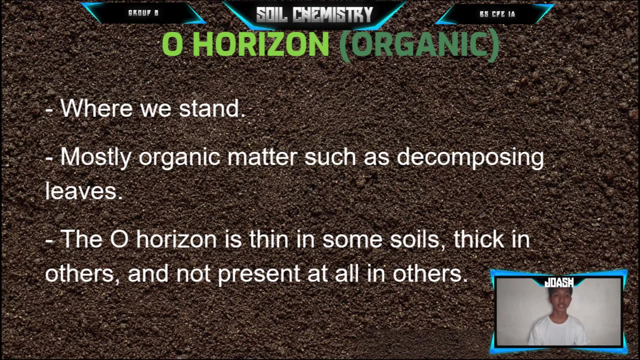 Soil is made up of distinct layers called horizon. They range from rich organic upper layers to underlying rocky layers. There are different types of soil layers and each of them has its own characteristics. And first I am going to discuss the O? horizon. first, The O? horizon is the top of all layers and 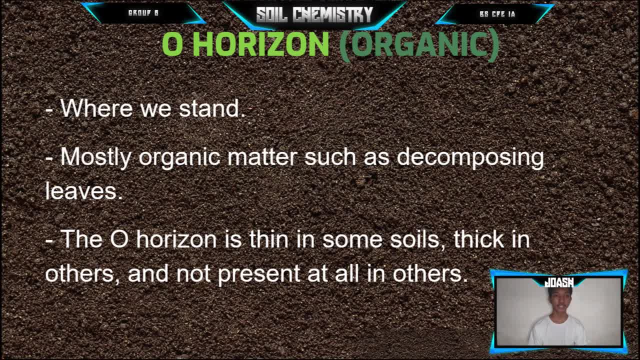 this is where we stand. This is the organic layer of soil and it is made up mostly of leaf, litter and humus, or which we call decomposed organic matter. The second layer is the A horizon. This layer is called the topsoil. It is found. 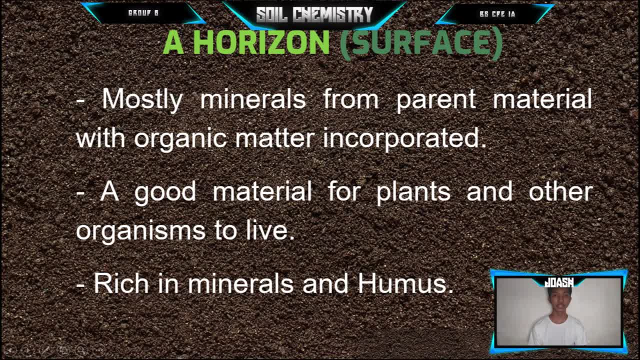 below the O horizon, Mostly minerals from parent materials with organic matter incorporated. This is where the seeds germinate and plants roots grow. It is a good material for plants and other organisms to live. It is rich in minerals and humus because it 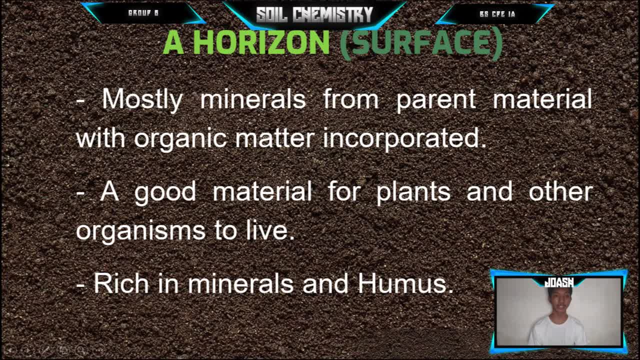 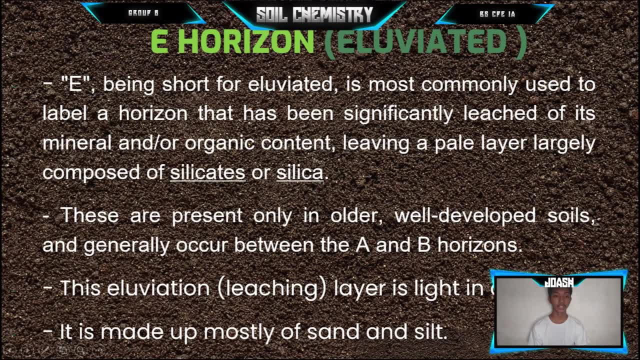 is made up of decomposed organic matter mixed with mineral particles. The third layer is the A-horizon. This alluviation layer is light in color. This layer is beneath the A-horizon and above the B-horizon. It is made up mostly of sand and silt, having lost most of its minerals and 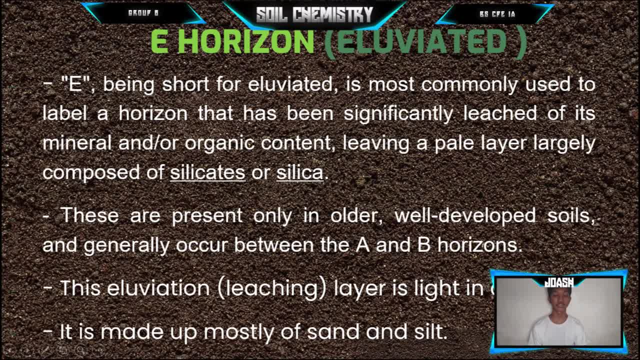 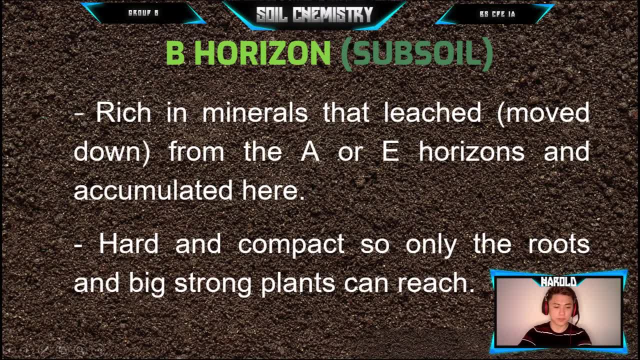 clay as water drips through the soil in the process of alluviation. And here is Harold Tongyo for the next layers. Next up we have the B-horizon, or known as subsoil. It is the layer of soil under. 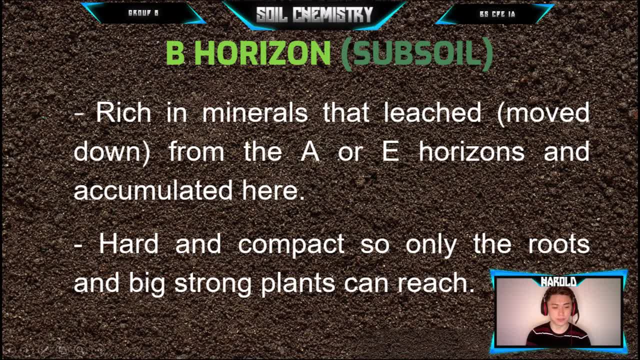 the topsoil on the surface of the ground. Like topsoil, it is composed of a variable mixture of small particles such as sand, silt and clay, But with a much lower percentage of organic matter and humus. subsoil can offer valuable nutrients and water for plant. 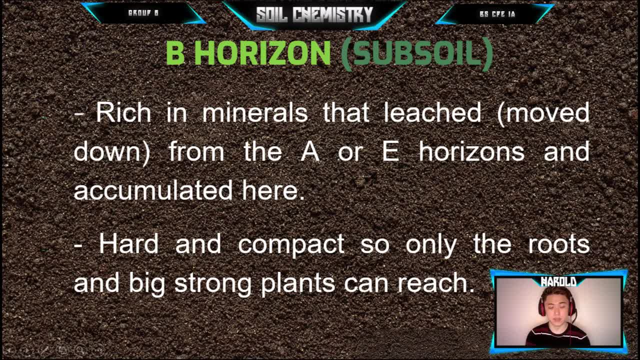 growth. Recent research has shown that, although nutrient availability to crops can vary, subsoil can contain a large share of the total nitrogen and phosphorus contained in the soil and retained water under drought conditions. Next up, we have the B-horizon. This alluviation layer is made up. 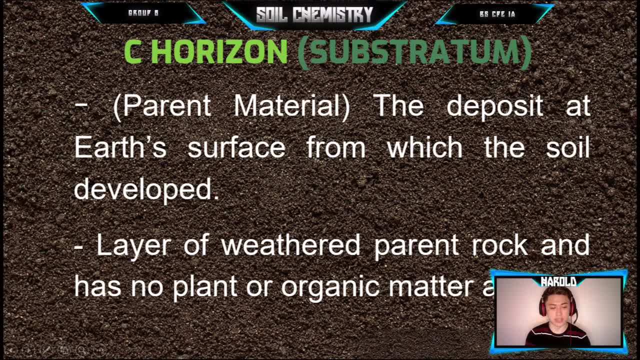 Next up is the B horizon. let's say, after the B horizon we have the C horizon, or for what we call the parent rock. Parent rock, also referred to as Subtratum, refers to the original rock from which something else was formed. It is mainly used in the context of soil formation, where the parent rock or the parent material 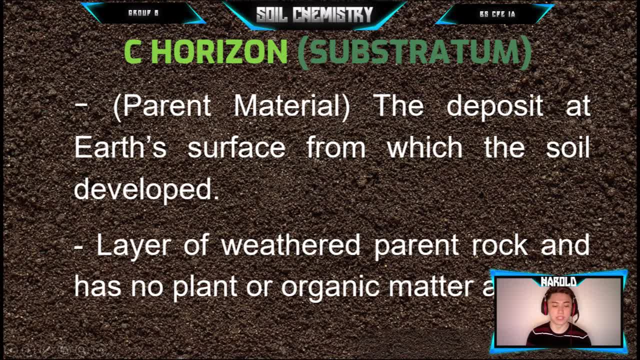 normally has a large influence on the nature of the resulting soil. For example, clay soil is derived from shale, while sandy soil comes from the weathering of sandstones. The term is also used in the context of metamorphic rocks, where again the parent rock, or potholith, 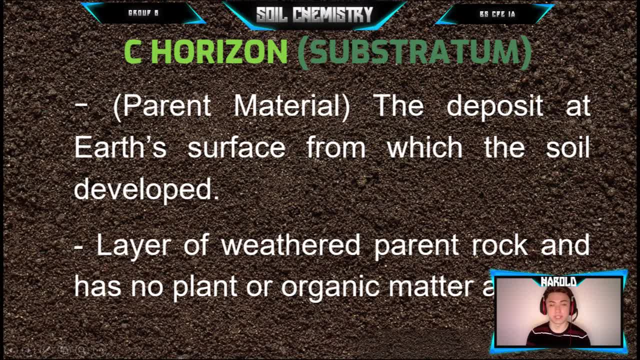 refers to the original rock before metamorphism takes place. Parent rock can be the sedimentary, igneous or metamorphic. So, for short, this layer contains much of the material That the soil was originally made from. it will contain rock fragments. 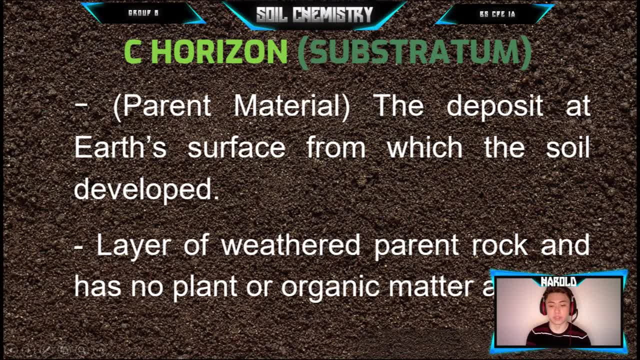 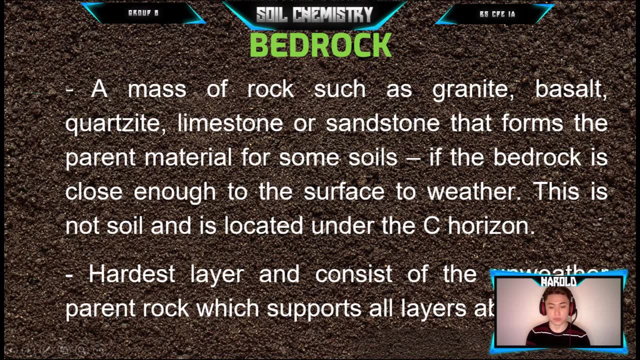 Weathering breaks down the parent rock into smaller and smaller pieces of rock, and this layer is most often light in color. And last is the R horizon or the bedrock. it is a massive rock such as granite basalt or quartzite, limestone or sandstone that form the parent material for some soil. 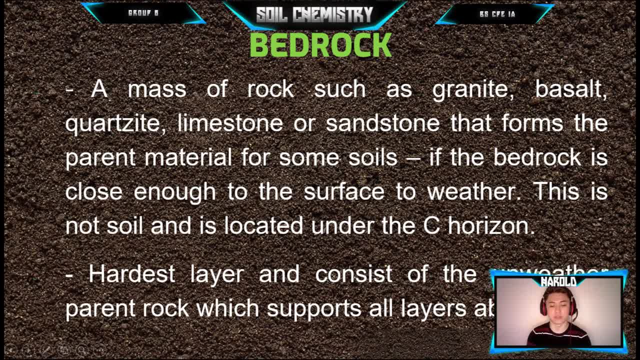 Bedrock can extend hundreds of meters below the surface of the earth towards the base of the earth's crust. The upper boundary of bedrock is called its rockhead or called rockhead. Above the rockhead, bedrock may be overlaid with sapphrolite. 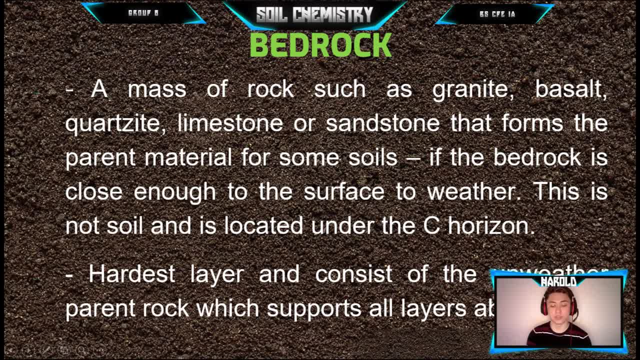 Sapphrolite is the bedrock that has undergone intense weathering or wearing away. Sapphrolite has actually undergone the process of chemical weathering. This means sapphrolite is not just less consolidated bedrock, it has a different chemical composition. 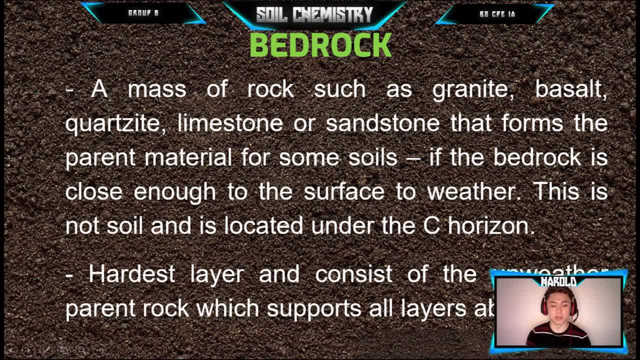 Flowing water or ice has interacted with minerals in the bedrock to change its chemical makeup. Above the sapphrolite may be layers of soil, sand or sediment. These are usually oak. They are often younger Unconsolidated rocks. 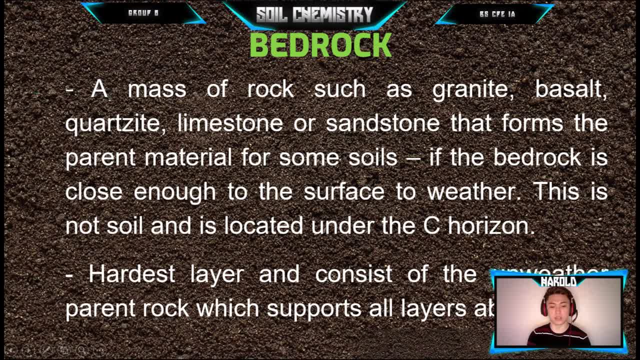 Exposed bedrock can be seen on mountain tops, along rocky coastlines, in stone quarries and on pages. Often these visible exposures of bedrock are called outcroppings or outcrops. Outcrops can expose through natural processes such as erosion or tectonic uplift. 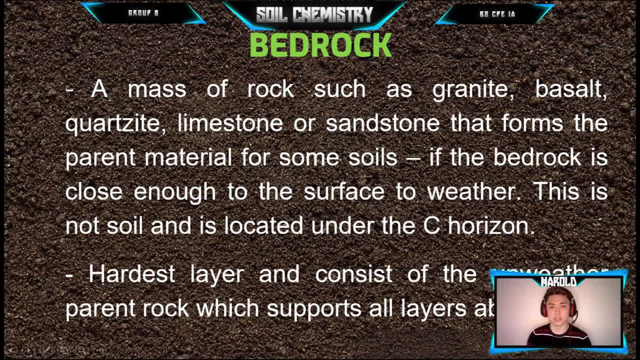 Outcrops can also be reached through deliberate outcrops. Outcrops can be exposed through natural processes such as erosion or tectonic uplift. Outcrops can also be reached through deliberate outcrops. Outcrops can also be reached through deliberate breathing. 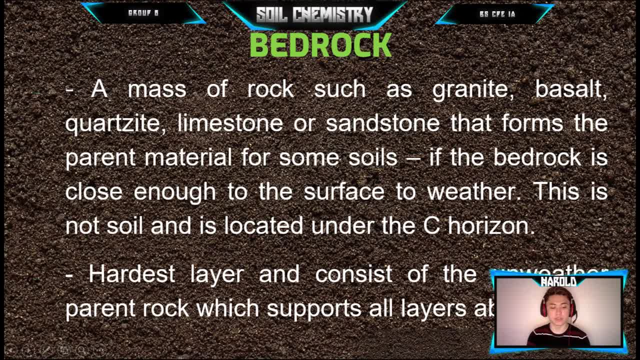 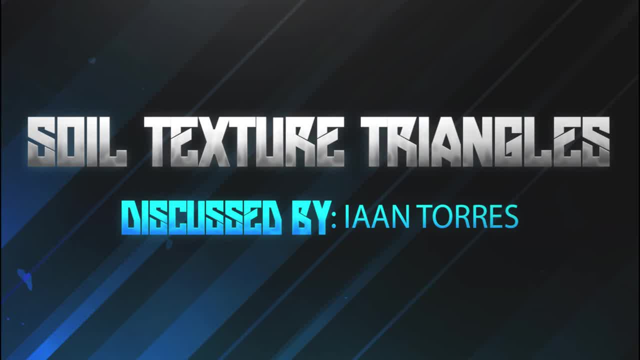 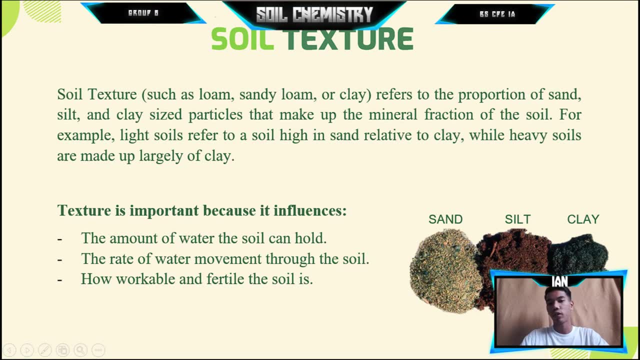 Outcrops can also be reached through deliberate breathing. Okay, so moving forward to Ian Torres to discuss the soil texture triangle. First of all, what is soil texture? What is soil texture? Soil texture refers to the proportions of sand, silt and clay sized particles that 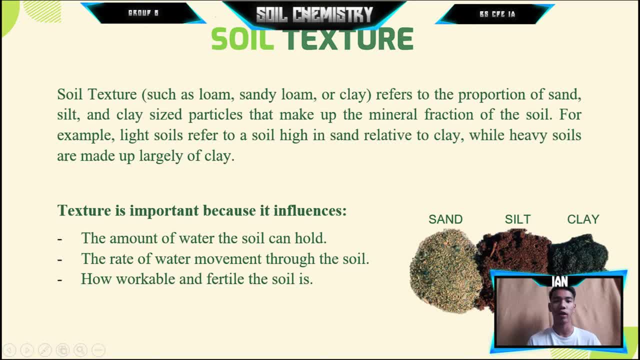 make up the soil. Why is texture important to the soil? Well, because it influences the following: Soil texture is a compound produced by soil. What is soil texture? The first one is the amount of water that soil can hold, and the second one is the rate of water. 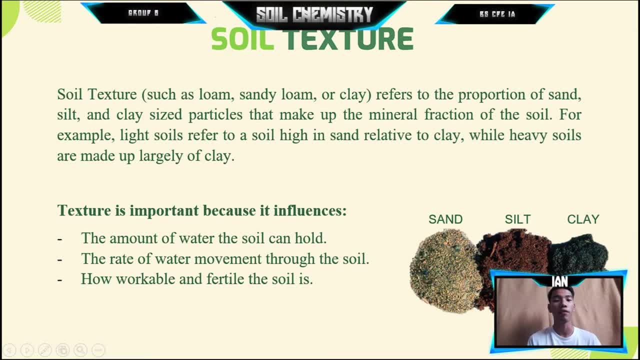 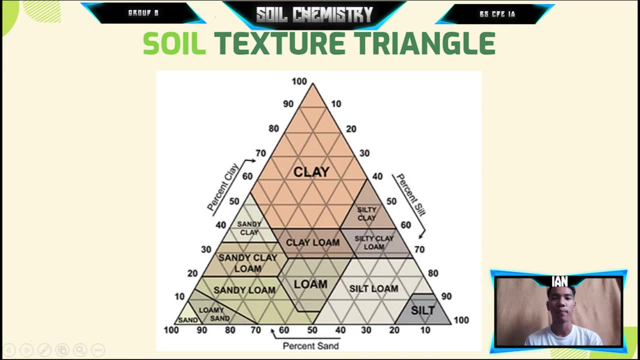 movement through the soil. and the third one is how workable and how fertile the soil is. Now let's go to the very complicated looking triangle. It is called the soil texture triangle. So looking at the triangle, it looks so complicated, but trust me, it wasn't. It was so simple. So the first thing you 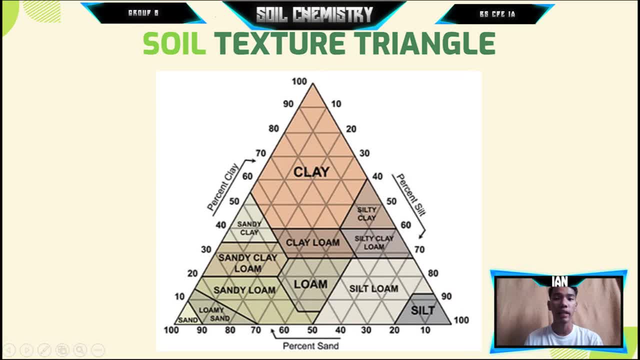 must do is to get the percentages of sand, silt and clay. So how will you do it? For example, you made your own mason jar soil test and you get these numbers. So how will you reflect these numbers on this soil texture triangle? So let's start in the clay side, but it depends on you. 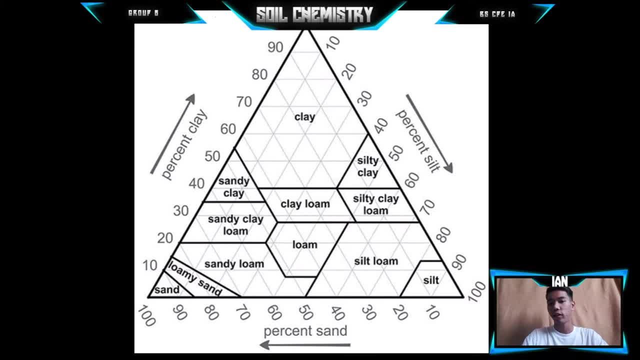 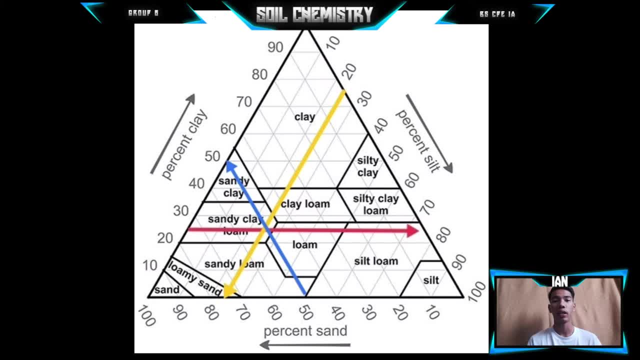 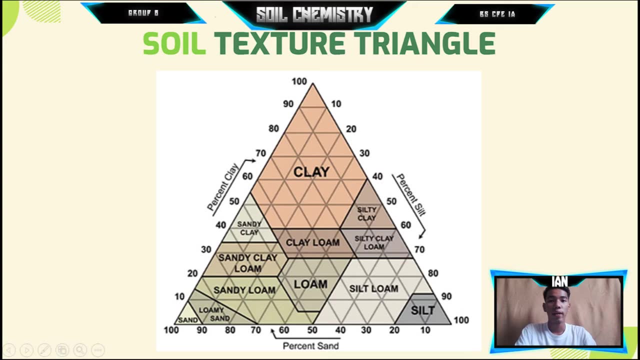 So, after reflecting the numbers we get from the sample jar soil test, we should take a look now where they intersect. So they intersect inside the piece of graph of sandy clay loam. So we can safely say that the type of soil in the sample soil test ends up being a sandy clay loam. So now let's proceed to. 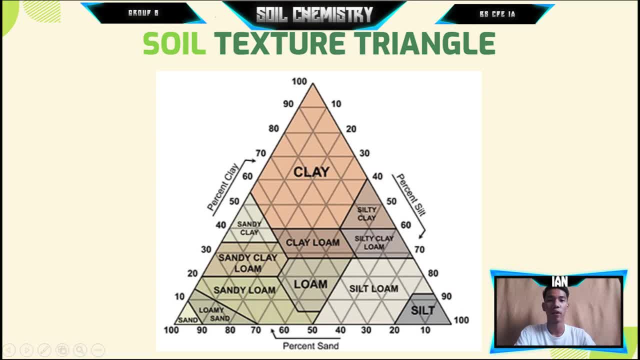 the soil texture to be discussed by Melvin. Once again, these are theunda, wildland, salt妈 silt, madwood sand silt, laid silt, variegated silt. Celtic silt, cladded silt clay. 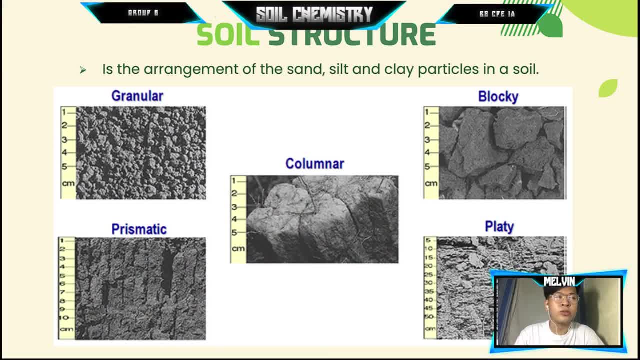 Next we have soil structure. Soil structure is defined by the way individual particles of sand, silt and clay are assembled: Single particles when assembled during a stronger particles. these are called arbitrary parts. The soil structure is the arrangement of sand with silt and clay particles granted to. 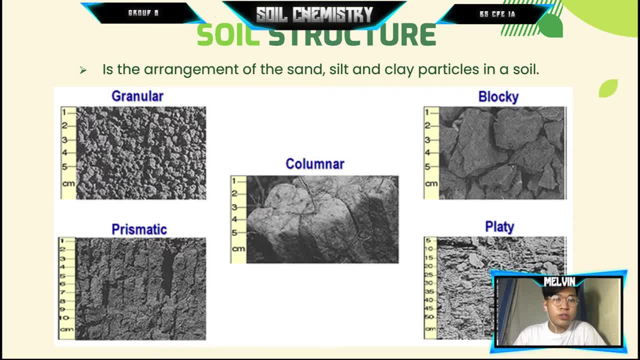 a group of people. And here when soil structure is defined by the way individual particles of sand, silt and clay are decent when enshrined, And here when sand is collected from the soil. We have different types of soil structure, for example, in our prismatic columnar, black and platy. 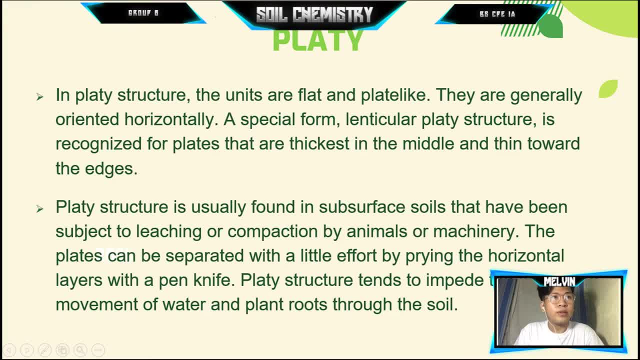 For season. In platy structure, the units are flat and plate-like. They are generally oriented. Resultantly, a special form of lenticular platy structure is recognized for plates that are thick, as in the middle, and thin toward the edges. The platy structure is made of salt particles that take a good place in thin plates or shapes, while horizontally 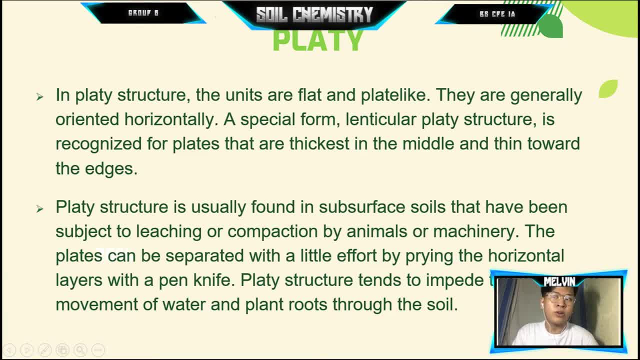 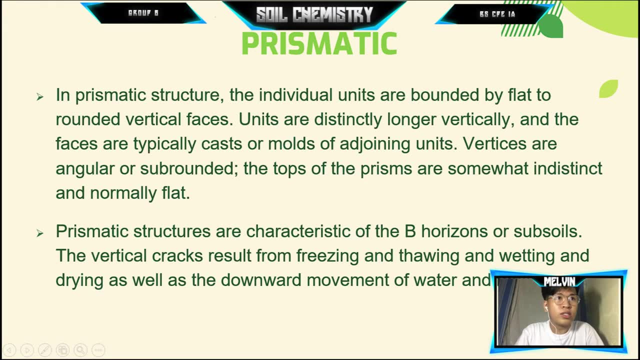 These plates often overlap. They have a big impact on water circulation. It is commonly found in forest soils and part of the day horizon, and in clay-like soils. Next we have prismatic- Prismatic structure. The individual units are bounded by flat to rounded vertical faces. 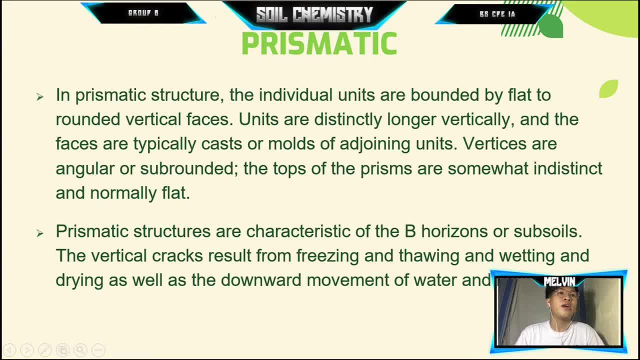 Units are distinctly longer vertically and the faces are typically cast or molds of conjoining units. Vertices are angular or so rounded. The tops of the prism are somewhat indistinct and normally flat. In prismatic the salt particles are formed into vertical columns or pillars. 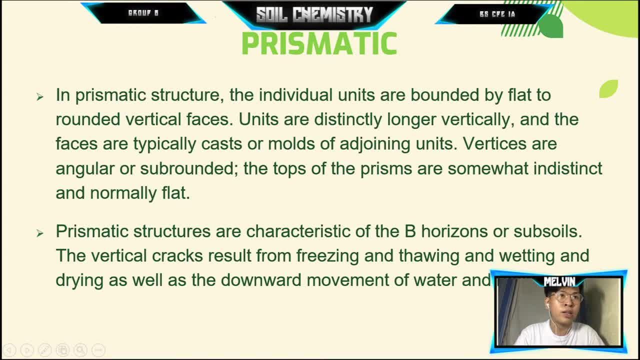 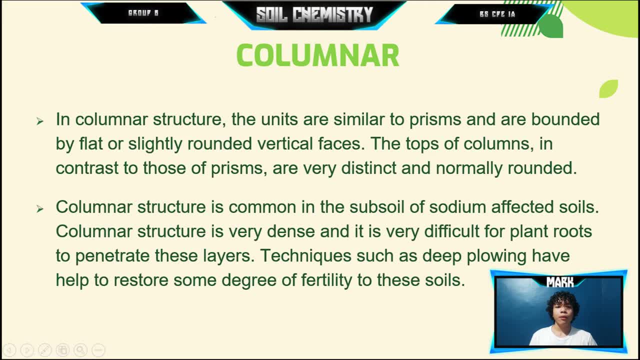 They can be seen in the B horizon where the plates are visible. Next we have Mark Vargas to continue the discussion about soil structures. Hi, I'm Mark Vargas. The next structure is columnar structure. In columnar structure, the units are similar to prisms and are bounded by flat or slightly rounded vertical faces. 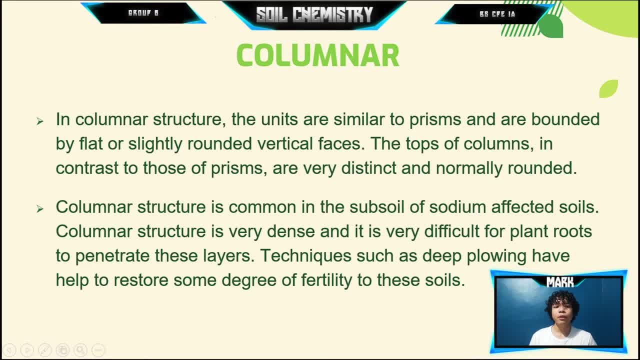 The top of columns, in contrast to those of prisms, are very distinct and normally rounded Columnar structure is common in the subsoil of sodium-affected soil. Columnar structure is very dense and it is very difficult for plant roots to penetrate these layers. 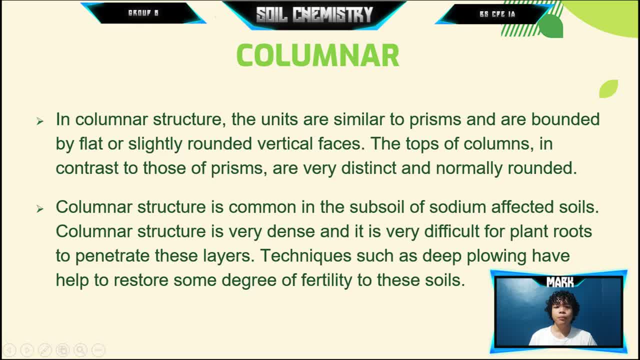 Techniques such as deep ploughing can help to restore some degree of fertility of these soils. It is where you have a lack of salt in your soil And what happens is the salt comes to the top layer of the prisms to disperse and sort of round off. 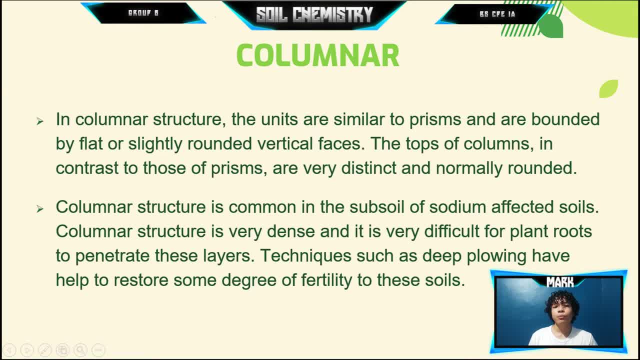 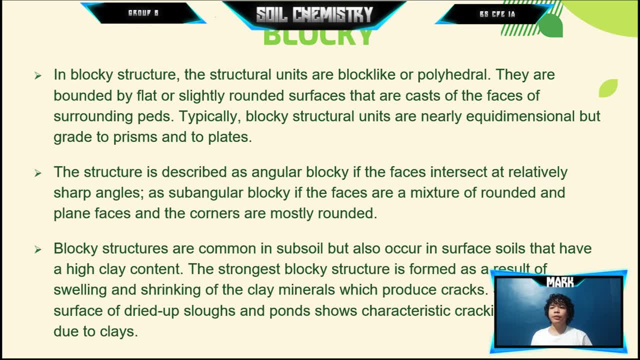 And you end up with what's called columnar structure. The next structure is block structure. In block structure, the structural units are block-like or polyhedral. They are bounded by flat or slightly rounded surfaces that are the cause of the faces of surrounding beds. 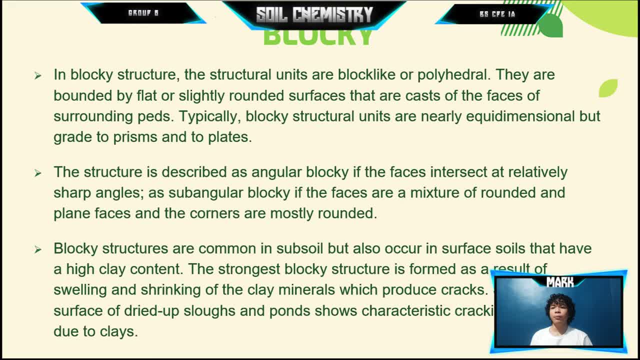 Typically, block structure units are nearly equidimensional, but great to prism and to plates. There are two types of block structure. The structure is described as this: It is described as angular blocky if the faces intersect at relatively sharp angles. As subangular blocky if the faces are a mixture of round and plain spaces and the corners are mostly rounded. 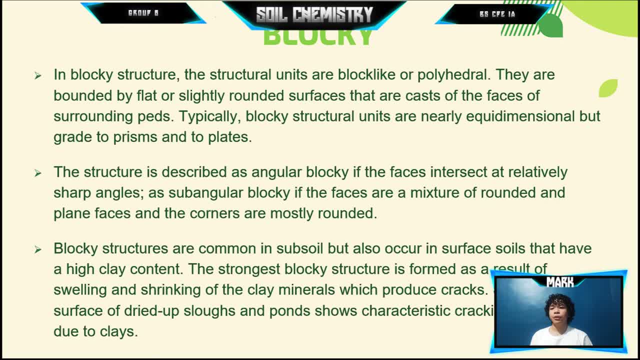 Block structures are common in subsoil, but also occur in surface soil that have a high clay content. The strongest block structure is formed as a result of swelling and shrinking of clay minerals, which produce cracks. The surface of dried axolotls and ponds show characteristics: cracking and peeling due to place. 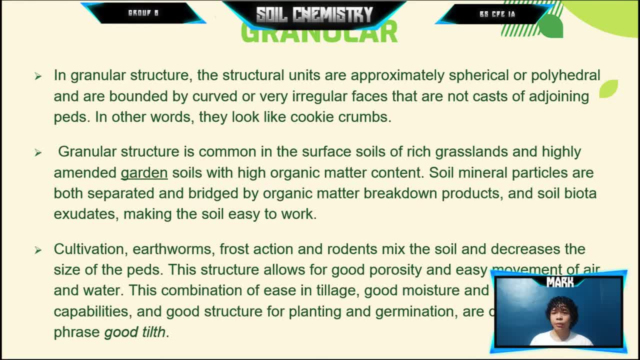 The next structure is granular structure. In granular structure, the structure units are approximately spherical or polyhedral and are bounded by curved or very irregular faces that are not cause of adjoining beds. In other words, they look like cookie crumbs. Granular structure is common in the surface of the soil of rich grasslands and highly amended garden soils with high organic matter content. 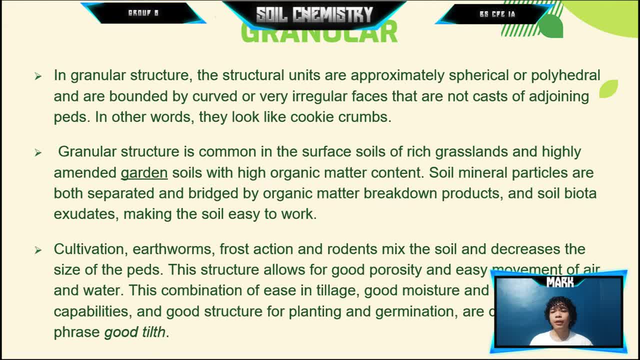 Soil mineral particles are both separated and rich by organic matter breakdown products And soil biota exudates making the soil easy to work. Cultivation, earthworms, frost action and rodents mix the soil and decreases the size of the beds. 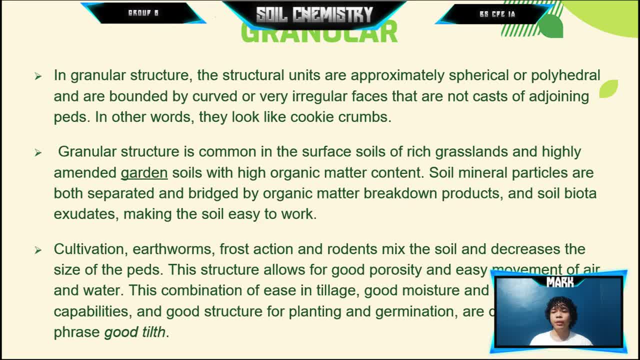 This structure allow for good porosity and easy movement of plants. This combination of ease in tillage and good moisture and air handling capabilities and good structure for planting and germination are definitive of the phrase good till With these fine particles which are actually stuck together by organic matter, it gives you good granular structure. 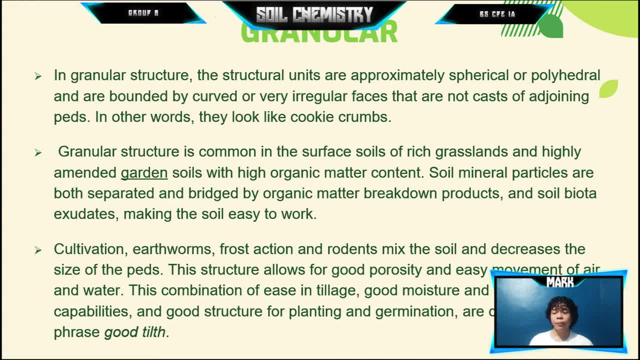 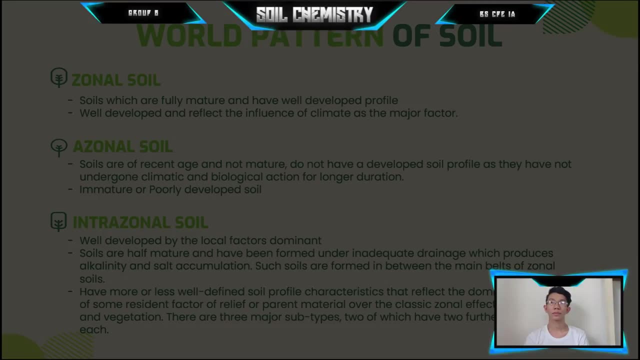 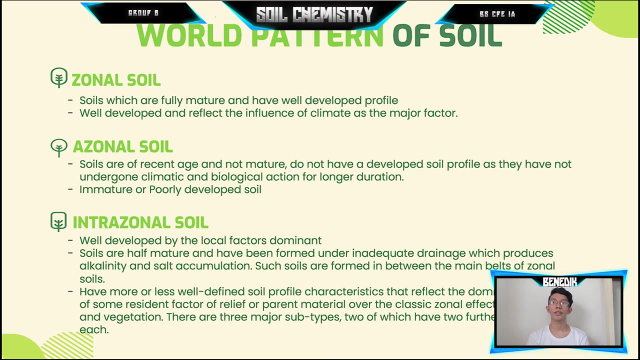 So the more organic matter that you have, the better your granular structure will be, And that's the five soil structure Moving forwards, let Christian Trinidad discuss the world pattern of the soil. Due to variations in soil texture, pH values, color structure and consistence, a variety of soils occur in the world. 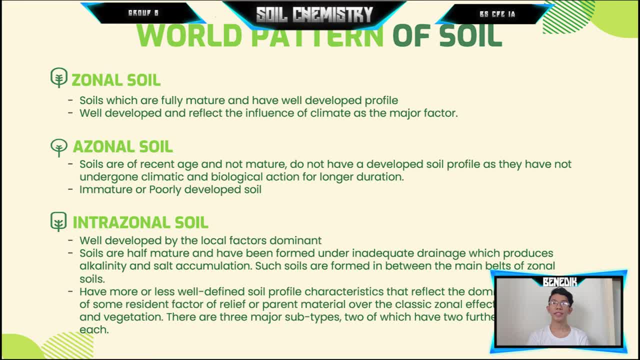 On the basis of maturity, These soils can be classified into three broad groups: Zonal soils, azonal soils and intrazonal soils. Zonal soils are soils which are fully mature and have well-developed profile. These soils reflect the influence of the regional climate and the vegetation that grows there. 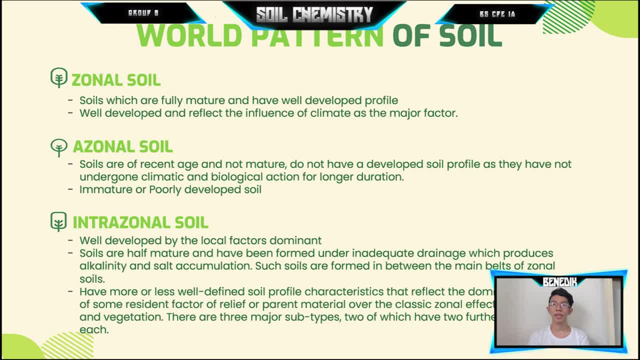 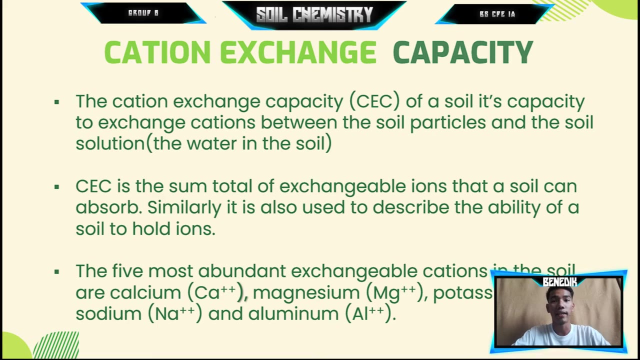 Azonal soils are soils of recent age and are not mature. These soils don't have a developed profile. They have not undergone climatic and biological action for longer duration. Unlike the zonal soils, Azonal soils are poorly developed soils. So what is cation exchange capacity? 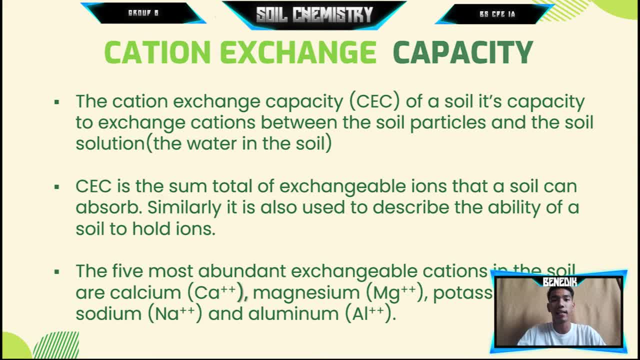 The cation exchange capacity of a soil is its capacity to exchange cations between the soil particles and the soil solution. So the cation exchange capacity is the sum of the total of exchangeable ions That a soil can absorb. Similarly, it is also used to describe the ability of a soil to hold ions. 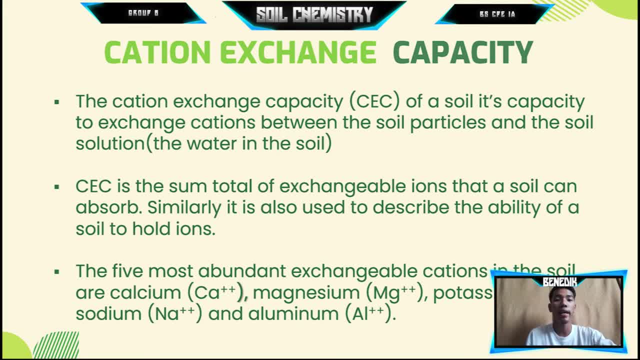 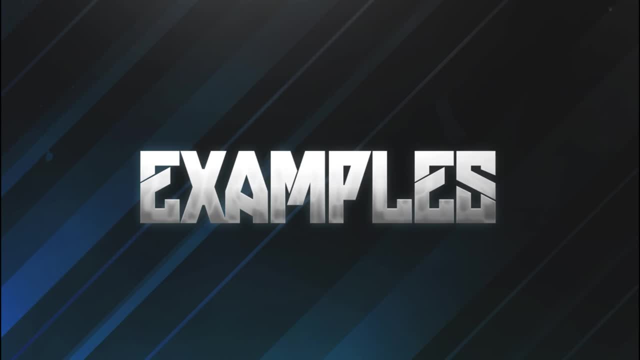 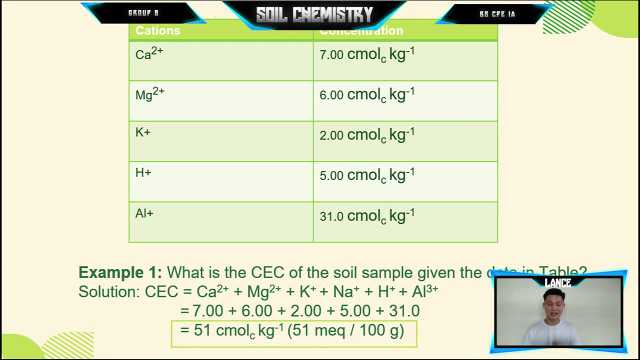 There are these five most abundant exchangeable cations in the soil, Which are calcium, magnesium, potassium, sodium and aluminum. So, guys, now let's move on to the first example, The first example of cation exchange capacity. So the given problem is: what is the cation exchange capacity of the soil sample, given the data in table? 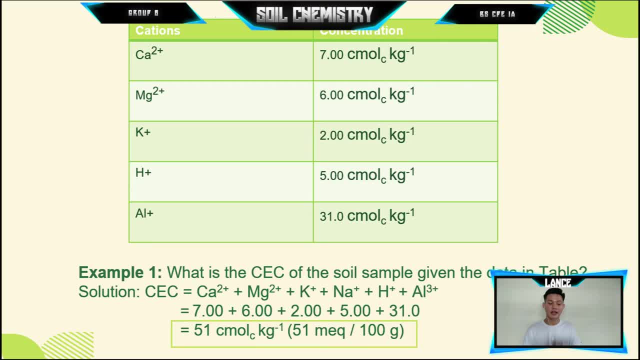 So now let's proceed in determining our given. So first we have calcium, squared with a concentration number of 7.00 cm2.. Followed by magnesium, squared with a concentration number of 6.00 cm2.. Followed by potassium with a concentration number of 2.00 cm2.. 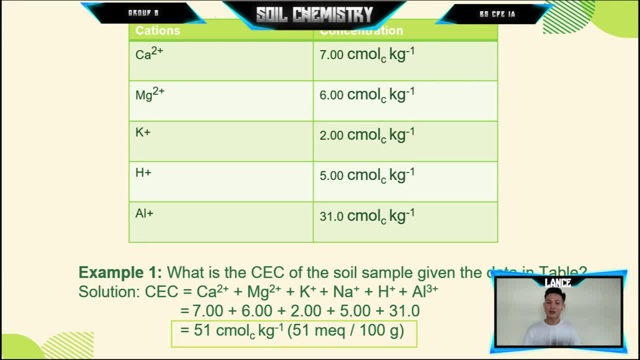 Followed by hydrogen with a concentration number of 5.00 cm2.. And lastly, we have aluminum with a concentration number of 31.0 cm2.. So, after knowing and getting our given, we are going to determine our solution. 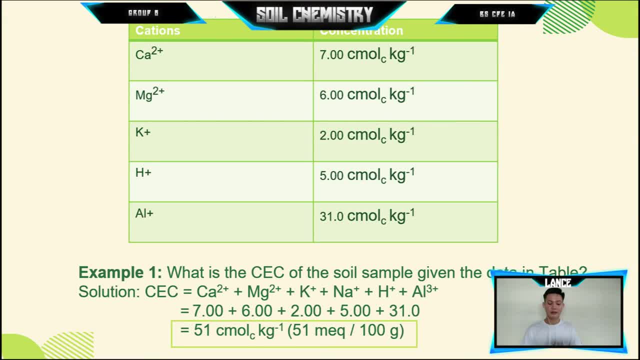 Our solution that we are going to use to solve this problem is: Cation exchange capacity is equal to calcium squared plus magnesium squared plus potassium plus sodium plus hydrogen plus aluminum. So, after knowing the solution and knowing the given, all we have to do is to substitute based on the value of our given. 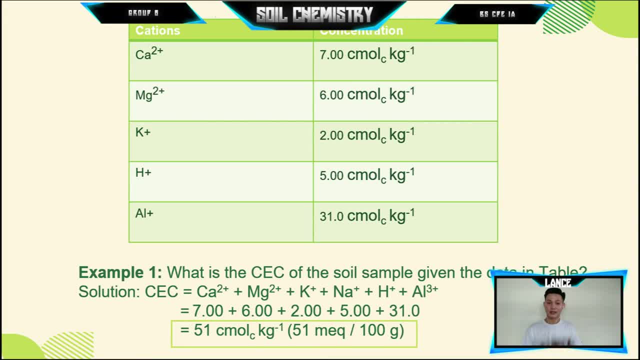 So our next step is to substitute. So for calcium, we are going to use 7.00 cm2.. For magnesium squared, we are going to use 6.00 cm2.. For potassium, we are going to use 2.00 cm2.. 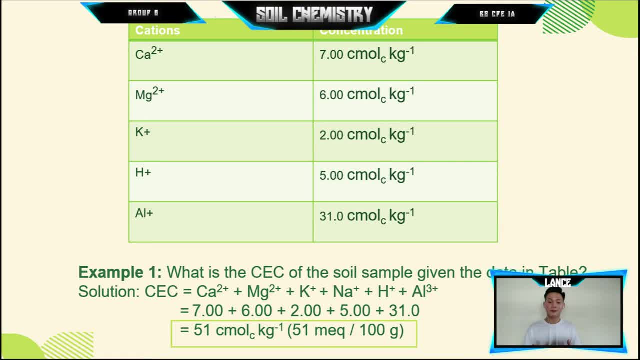 And for sodium. as you can see, guys, the sodium is not a part of the data given in the table, So what we are going to do is we are going to cancel it out because its value is 0.. Next one is hydrogen, with a value of 5.00 cm2.. 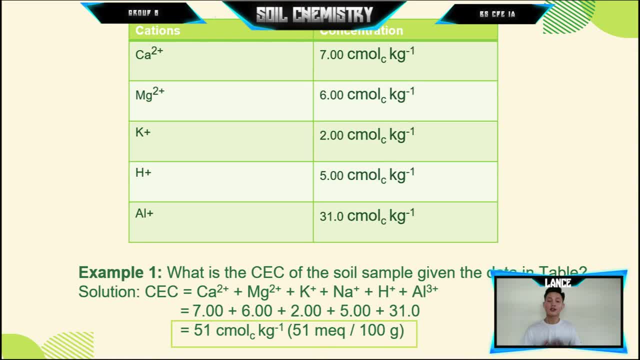 And aluminum with a value of 31.00 cm2.. So, after we substitute, all we have to do is to add those values And we are going to come up with an answer of 51.00 cm2 of charge. And then, after that, guys, if we are going to go back to the first table, 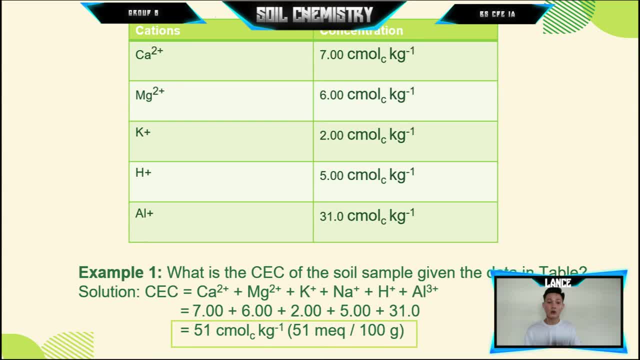 we will see that the first example is in the soil-competent: more molybdenum clay and smectite clay, Because the 200 and the 150 is greater than 51. And then the 30 below is less than 51.. 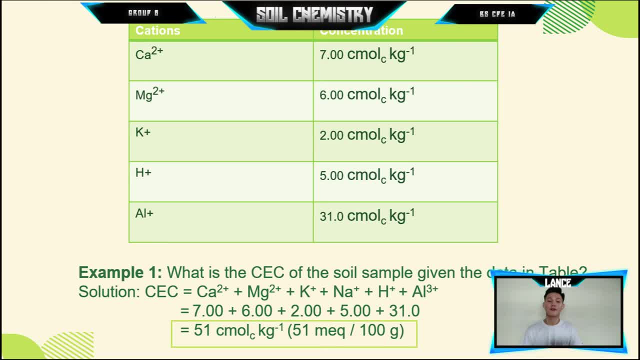 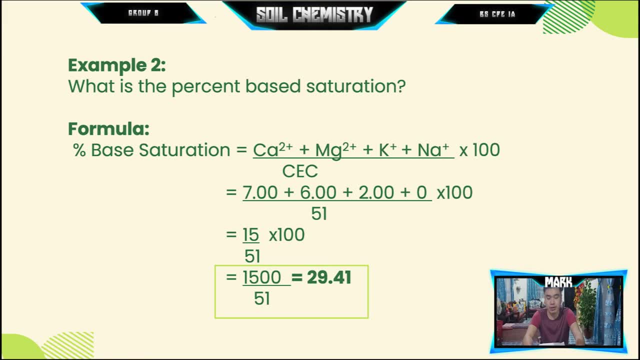 That is why our first example is, in the soil-competent, more molybdenum clay. Let's go to example number 2.. What is the person-based irritation? Person-based irritation is the percentage of the CD occupied by the basic cations. 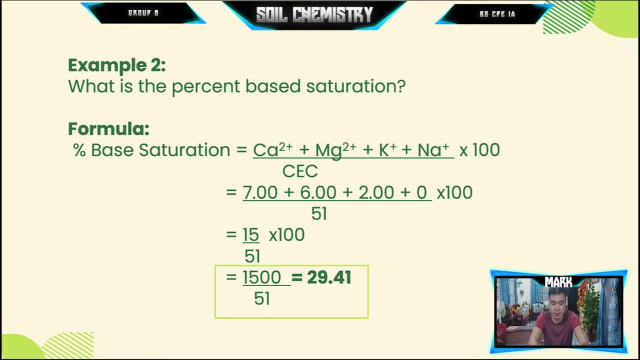 of calcium with the base of 2-phosphate, magnesium with the base of 2-phosphate and potassium-phosphate. The person-based irritation is the percentage of the CD. What is the CEC? The CEC is the Cation Exchange Capacity. 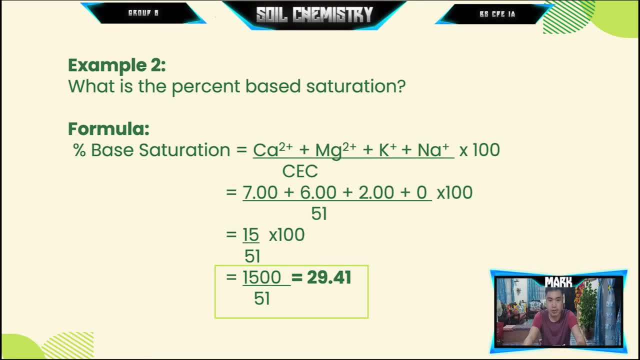 This is the quality of the soil that is occupied by the exchangeable cation. The CEC is also the one that influences the soil, that also occupies the nutrients and provides the soil solidification. So we have a problem here. What is the formula of the person-based irritation? 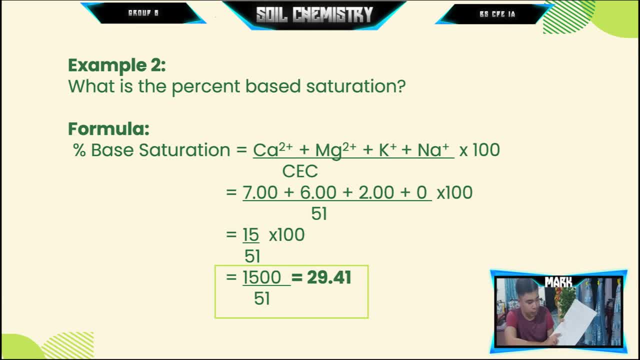 This is the formula of the person-based irritation. Ca is the base of 2-phosphate plus magnesium, with the base of 2-phosphate plus potassium-phosphate plus Na-sodium plus times 100.. So how is the person-based irritation solved? 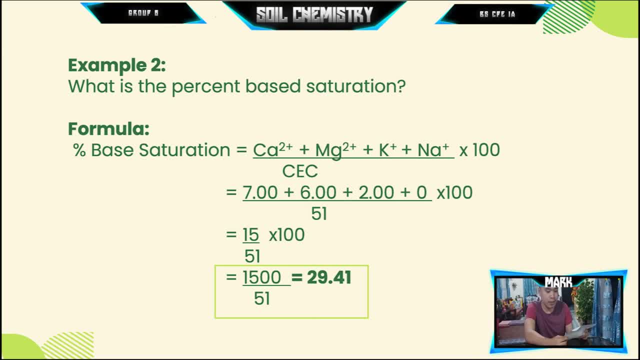 To calculate the person-based irritation, divide the sum of the given, then multiply it by the 100%. First, add the sum of the given, then multiply the result by 100%. So this is the given Ca squared plus Mg squared plus 8 plus. 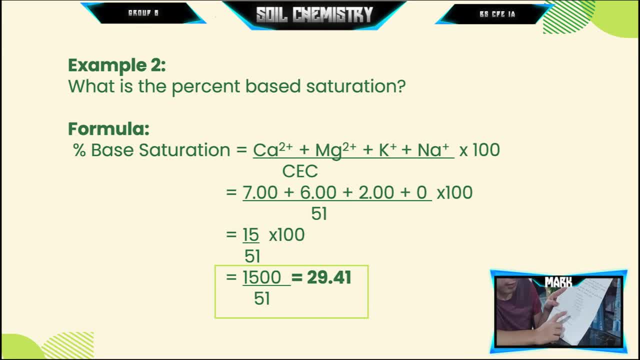 positive plus Na, plus positive times 100 over CEC. So to get this, we will just convert this to the given in the chart. So what is calcium with the base of 2?? That is 7.00.. That is what is written in our chart. 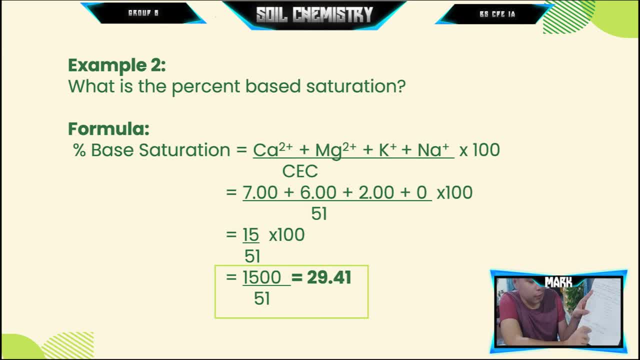 We will just follow our chart: Plus 6.00, plus 6.00, plus 2.00, plus 0 times 100 over 51.. Where did we get the 51?? We got the 51 in the example number 1.. 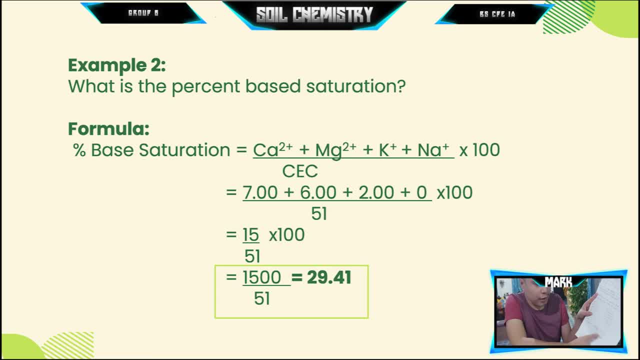 So let's proceed. We will just add this: This 4 will be 15.. We will just rewrite the times 100 and the 51. Over 51. So we will just multiply the 15 by 100.. We will get 1,500. 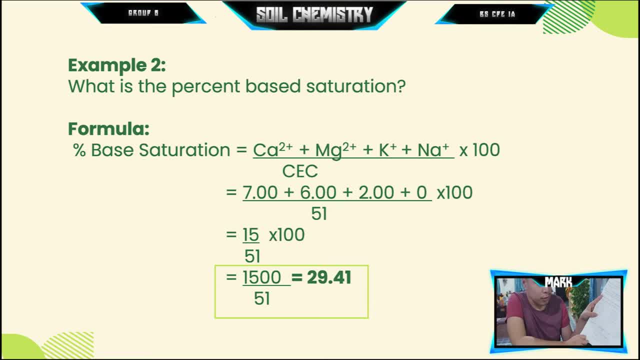 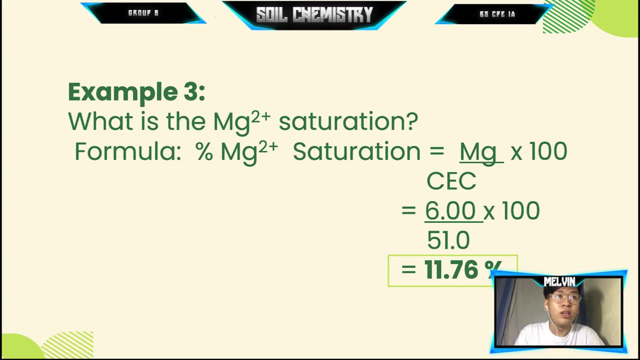 We will just rewrite the over 51. So here we got 1,500 over 51. We will just divide this. We will get the answer, which is 29.41.. Next we will get the concentration of the magnesium to positive. 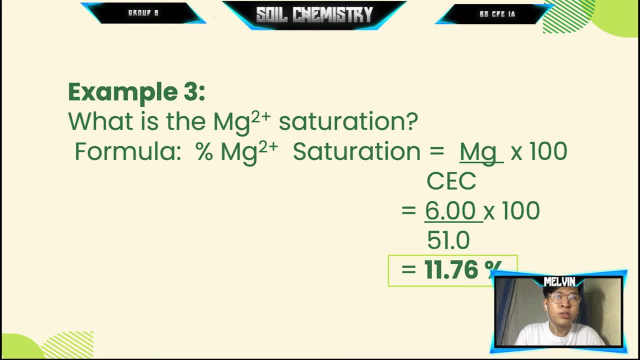 We can see in the table that the concentration of the magnesium to positive is 6.00.. And our CAC is 51. We will just divide 6 by 51. Then times 100, we will get 11.76%. 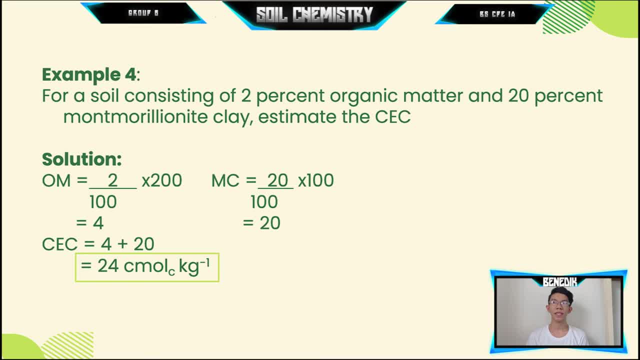 For our last example on calcium exchange capacity. we have this problem For a soil consisting of 2% organic matter and 20% montmorillonite clay. estimate the calcium exchange capacity For this problem. we are given the percentages of two soil components. 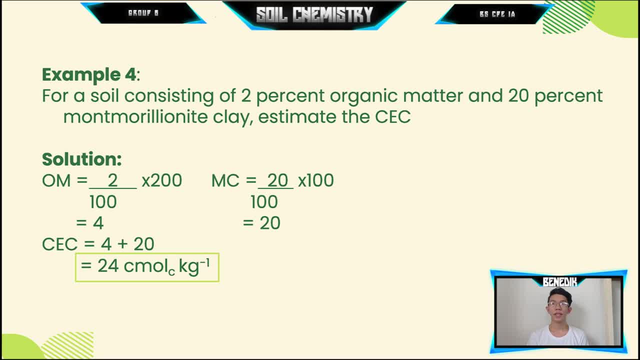 These are 2% organic matter and 20% montmorillonite clay. We are required to find the sum total of exchangeable ions that this soil can absorb, or its CEC. To find its total CEC first we need to solve the CEC of each individual soil component. 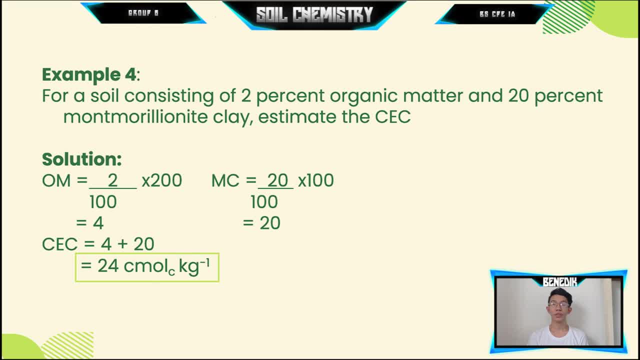 For the organic matter, we multiply 2%, which is 2 over 100 by 200, which is the approximate CEC of organic matter, and we will get 4.. Next, for the montmorillonite clay, we multiply 20%. 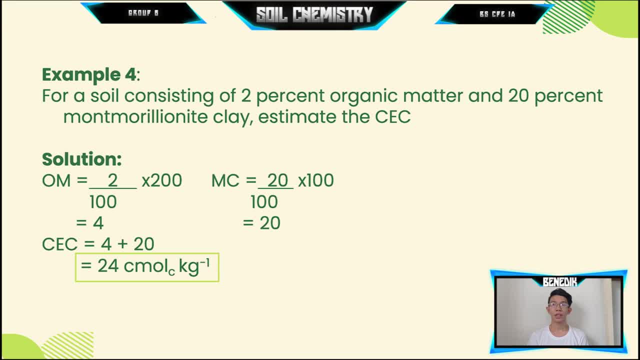 which is 200 by 100, which is the approximate CEC of montmorillonite clay, and we will get 20.. After solving the CEC of each individual soil component, we need to get its sum to know the total CEC. So 4 plus 20 would give us the answer 24.. 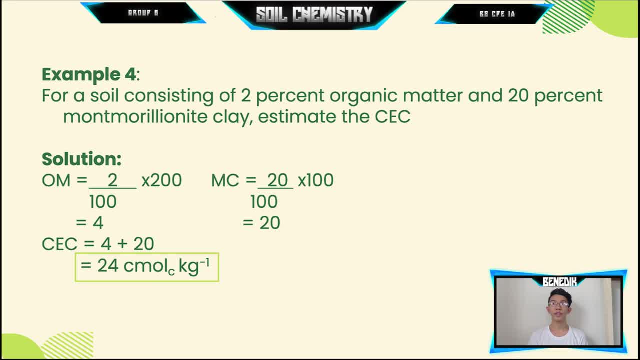 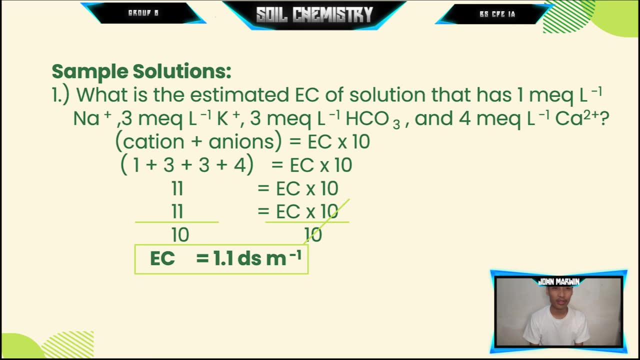 So this soil has a calcium exchange capacity of 24 centimoles of charge per kilogram. Hello guys, I am Delmarine Sumang and I am here to discuss the sample solution number 1.. Sample solution number 1.. What is the estimated EC or electric conductivity of solution? 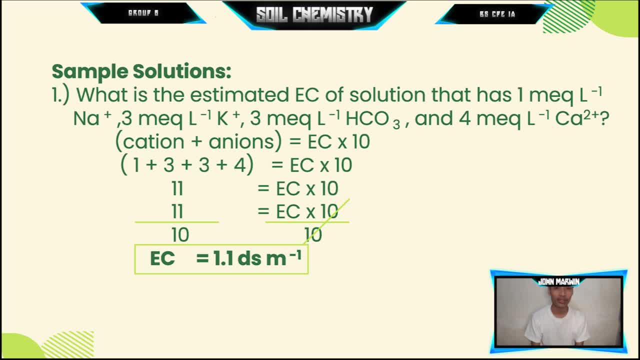 that has 1 milliequivalent per liter of sodium ion, 3 milliequivalent per liter of potassium ion, 3 milliequivalent per liter of bicarbonate ion and 4 milliequivalent per liter of calcium ion. 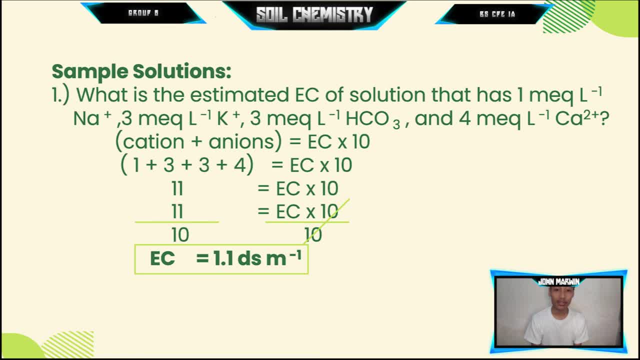 In this sample question, the missing value that we are going to find is the EC or the electric conductivity. In order to get the answers, we need to use this formula: Cations plus ions is equal to EC multiplied by 10.. First, we need to gather all the given in the problem. 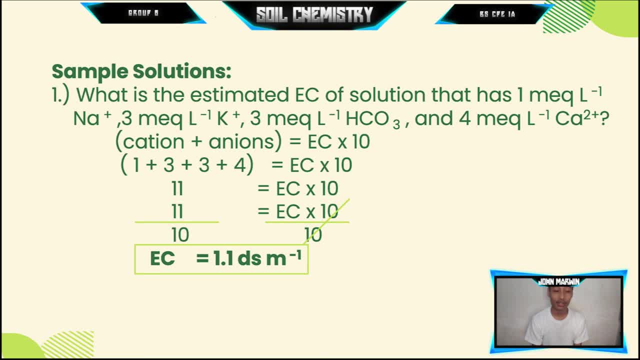 These are the 1,, 3, 3 and 4.. In the formula we need to add all the cations and the ions, and that is: 1 plus 3 plus 3 plus 4 is equal to EC multiplied by 10.. 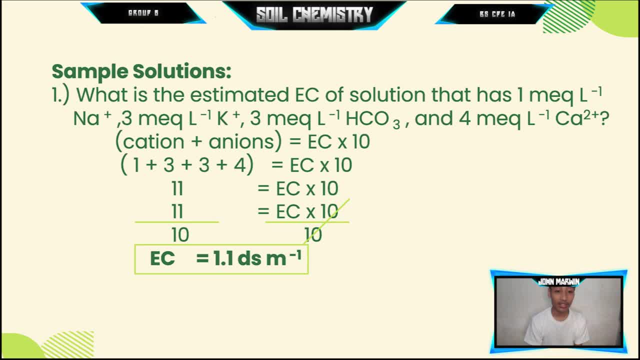 And we will get the answer of: 11 is equal to EC multiplied by 10.. Since the missing value is the electric conductivity, we need to divide both sides by 10 in order to cancel the 10.. The last step is divide 11 by 10. 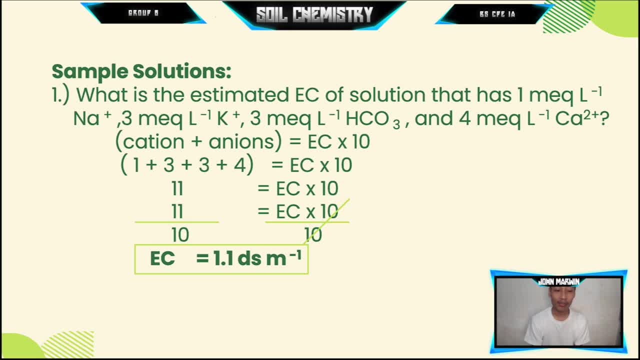 and we get 1.1.. Therefore, in the problem the electric conductivity that is missing is equivalent to 1.1 desiccantions. And here is Jan Emil Torres for the next sample question. Hi, I'm Jan Emil D Torres. 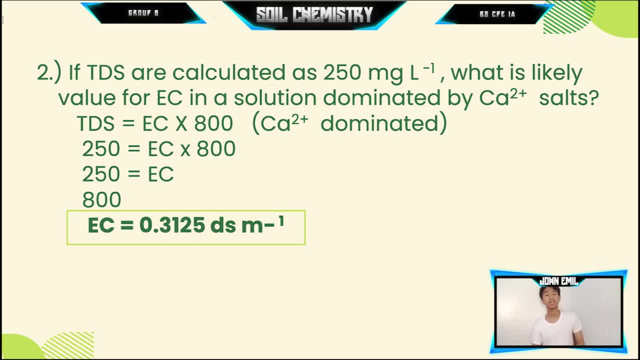 and I'm here to discuss the sample number 2.. If total dissolved solids are calculated as 250 mg per liter, what is likely value for electrical conductivity in a solution dominated by calcium ion salt? So in this problem we need to find the easy solution. 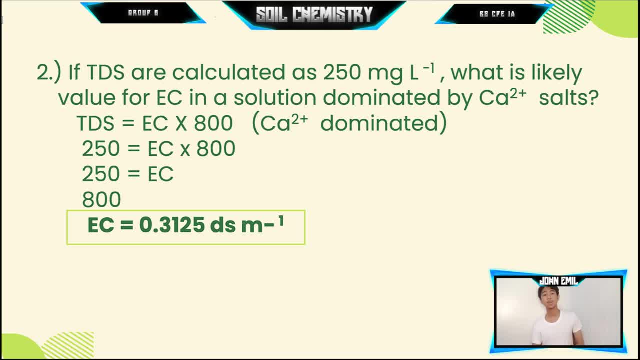 dominated by calcium ion salt. So we will use the formula: total dissolved solids is equal to electrical conductivity times 800, which is the calcium ion is dominated And the TDS is given. It is 250 mg per liter and is equal to electrical conductivity times 800.